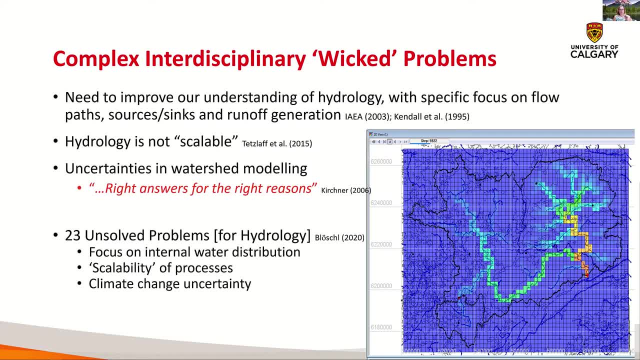 And so for that we really need to make sure that we have the correct soil moisture if we want to mimic the correct evapotranspiration. So we need the water in the right place, And this really comes back to Gunter Blaschel's paper 23: Unsolved Problems for Hydrology. 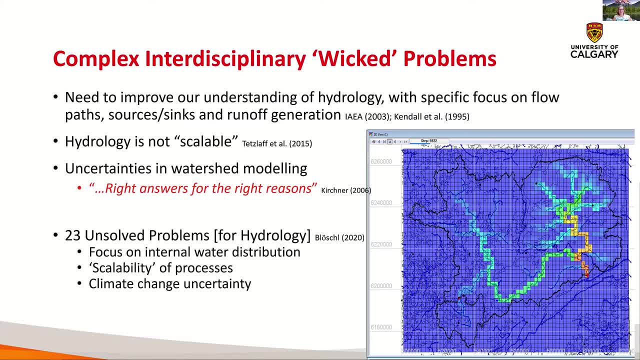 If you haven't had a chance to check out that paper, especially for the students online, I really suggest that you do, because it really underpins nicely some of the thrusts that need our attention and our focus, including looking at internal water distribution in models, scalability of processes and climate change uncertainty, all of which I'll address at some point in this presentation. 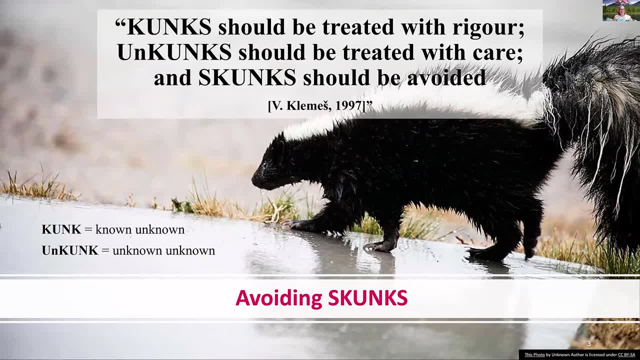 So this is one of my favorite quotes: Cunks should be treated with rigor, Uncunks should be treated with care and skunks should be avoided. This came from Vic Clems- he was. he borrowed the terminology from military tech, military terminology. 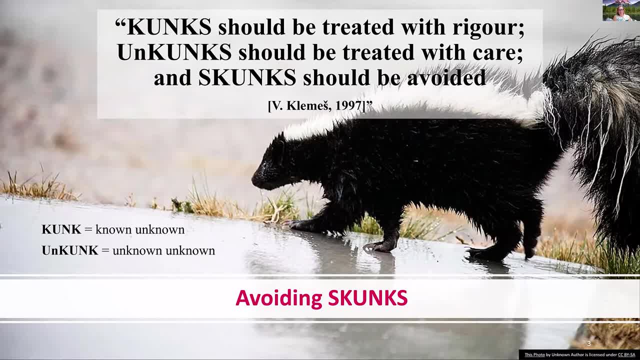 But he was a famous hydrologist that worked for the government of Canada for many decades actually, And the idea here is to basically suggest that we have to accept that there's going to be known unknowns, things that we're actually planning for, and uncertainty analysis. 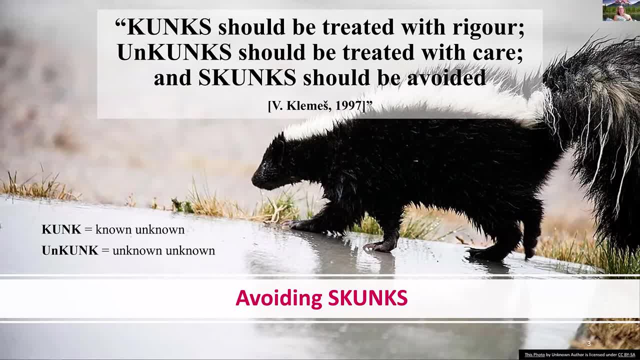 We know that our input data introduces some uncertainty, So we explore that. But I think we sometimes forget that there's still unknown, unknowns And if you don't plan for that as a modeler or account for that, then you're pretty much opening yourself up to some criticism there or some smelly situations, skunks. 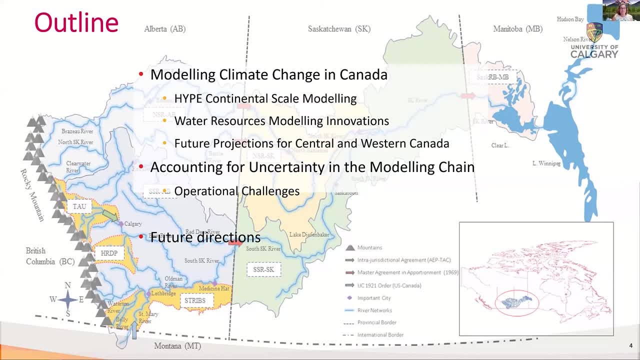 Okay, so the thrust of what I'm going to talk about today. I've broken into three main sections. First of all is to introduce you to some of the modeling that we're doing in Canada, particularly looking at climate change. I'll introduce you to the height model which we've been using at the continental scale. 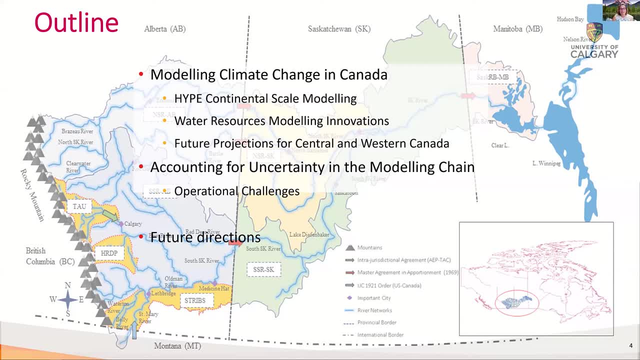 Talk about some water resources management modeling that underpins some of our work and helps to address some uncertainties, and then some of our future projections, Focusing mostly on Western Canada, because that's in large part the region that I've focused on, And there's good reason for that. 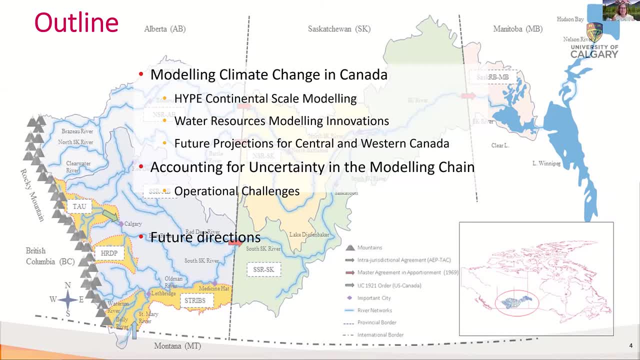 It happens to be where the most uncertainty is, which I'll also talk about. Then I'll talk about accounting for uncertainty in the modeling chain. So some of the things that we're doing to try to address both the skunks or the unkunks and the kunks. 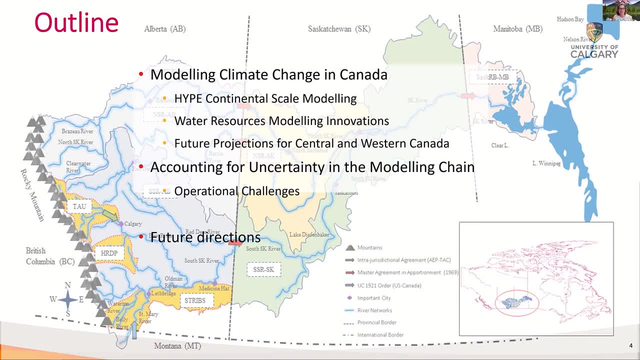 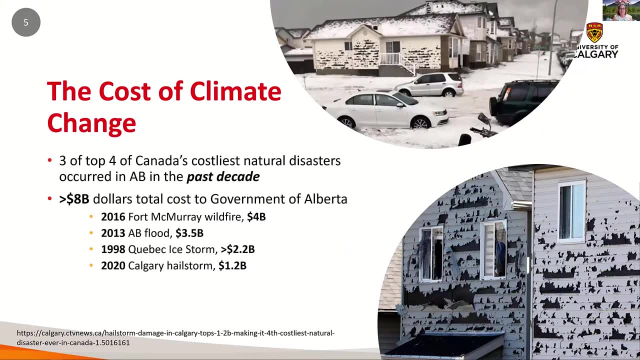 And then some future directions that I think we can integrate into Abinet. So for some context, Western Canada has been a large focus and this kind of summarizes why Three of the top four costliest Canadian natural disasters have occurred in Alberta within the past 10 years. actually, 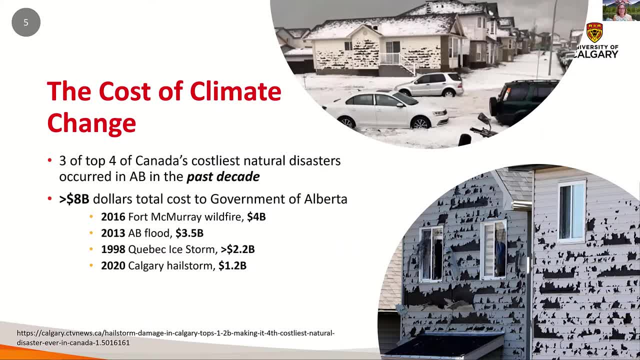 And maybe not a big surprise because costs go up over time, but they're pretty significant. More than eight billion dollars in total has been incurred. Cost has been incurred to the government of Alberta And I've summarized the most costly events here that have occurred within Canada. 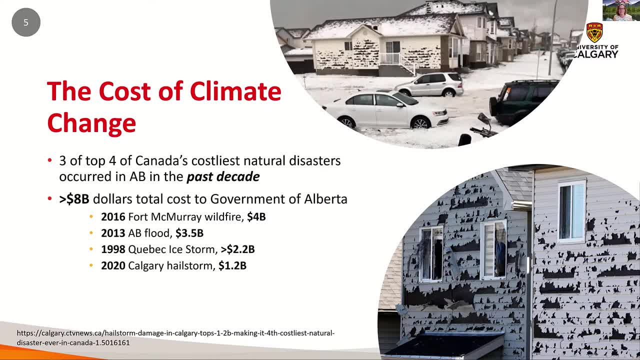 There's also the Quebec hailstorm in 1998. that was of significant concern. So we know it's not Not even a debate. We know that climate change is happening and we know that this is leading to some costs that we have to account for within our economy. 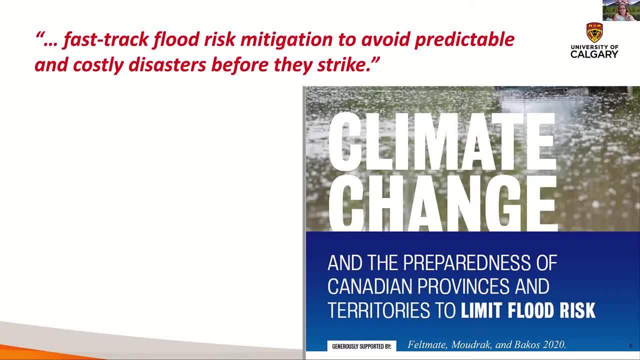 There was a report that was done by the Intact. Intact is an insurance company in Canada and they've sponsored- this should tell you everything. an insurance company has sponsored- a research institute within the University of Waterloo to look at the cost of climate change and how prepared Canadian jurisdictions we are. 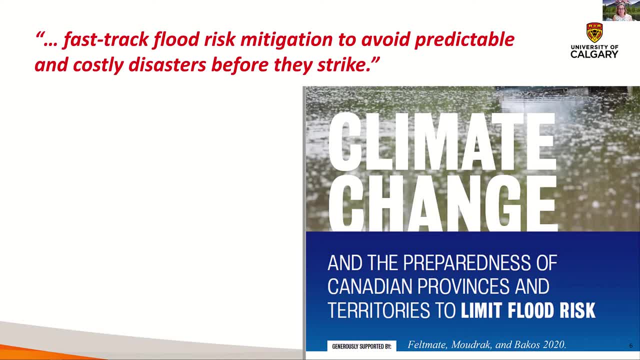 We were unfortunately given a grade of C across Canada. So you know, by my academic standards, not what I aimed for. And the insurance industry has outright stated that provinces and jurisdictions in Canada have a fiduciary responsibility to act. Otherwise they are liable. And that's pretty telling because insurance companies 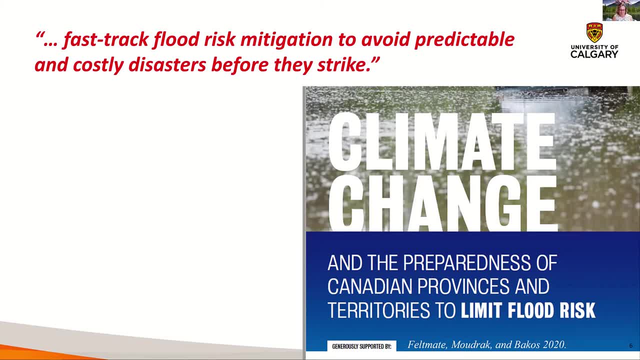 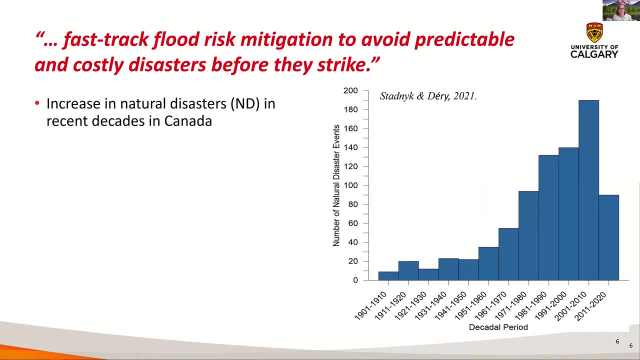 are no longer willing to actually support or pay out during these claims. This is from a paper that I published- this spring actually- and it shows the increase in natural disasters that have occurred in Canada in recent decades. So I broke it down by decade. 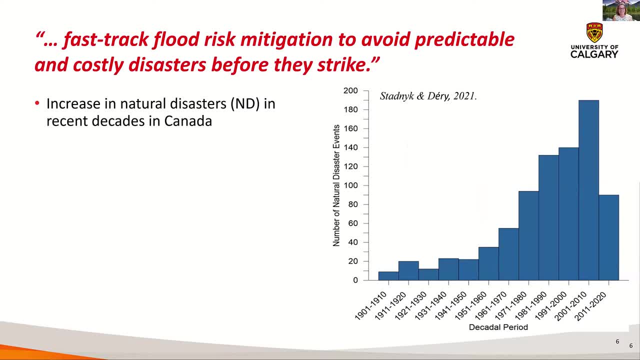 And this kind of distribution can be fit with an exponential model pretty easily. And although there's some questionability about earlier decades how well the reporting was in comparison to the reporting now, even if you account for that, there's still been a significant increase. 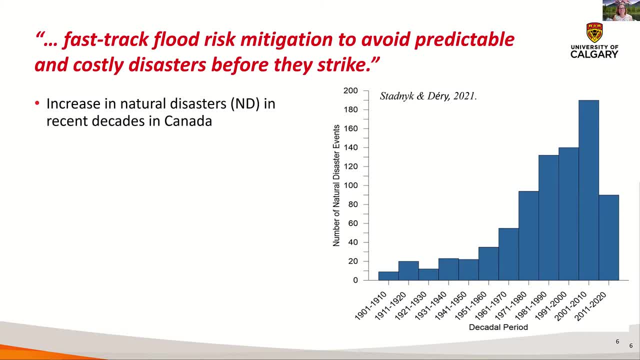 And the reason why the last bar isn't as high is because they hadn't finished updating the database. So this is from the Canadian, from Public Safety Canada, the Canadian Natural Disaster Database, And if you actually break this down a bit further, you can see that a significant number of the natural disasters 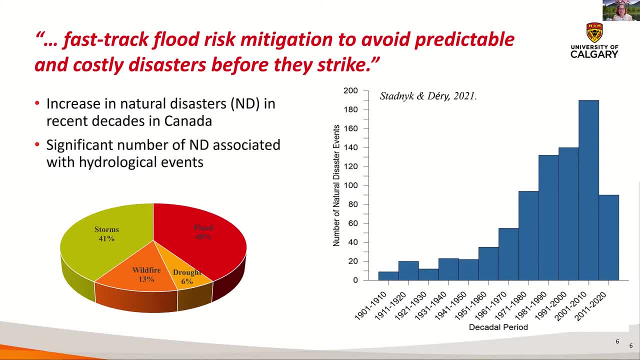 are associated specifically with hydrology and hydrological events. So there's the obvious one, flood, which makes up about 40% of these natural disasters, but arguably drought and subsequently wildfire in drought years are also associated, at least in part, with hydrometeorology and certainly storms. 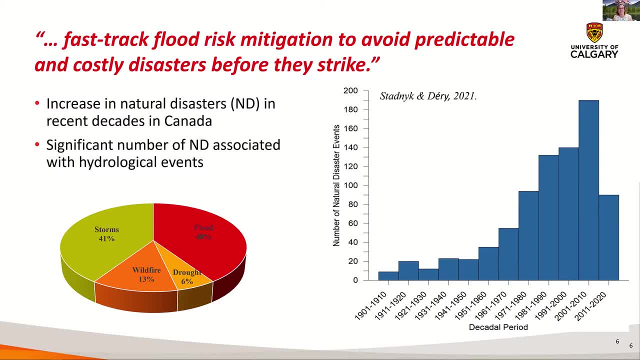 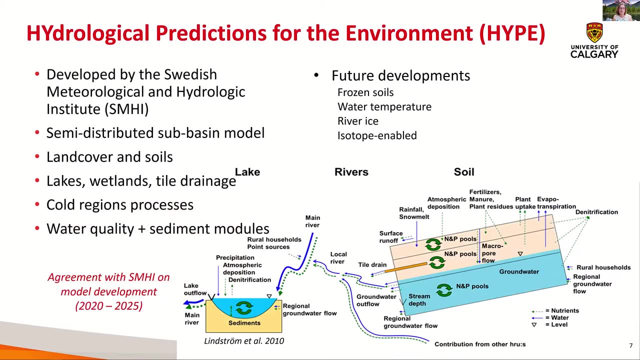 So there's a significant percentage of these events that can be tracked or attributed to how we look at water on the landscape. So the model that we are using right now for our continental scale prediction is the HYPE model. It's developed by the Swedish Meteorological and Hydrological Institute, or SMHI. 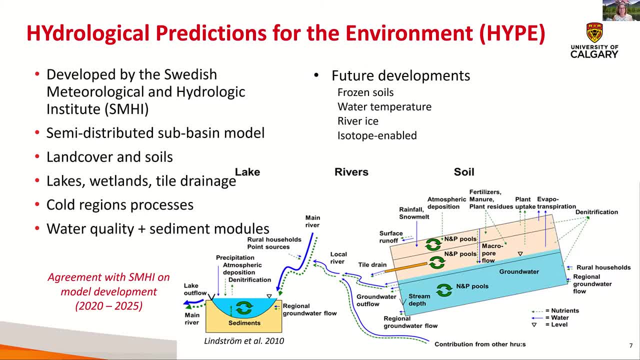 Some of you might already be very familiar with this model. It is used operationally across Europe. It's a semi-distributed sub-basin model. So I call it semi-distributed because it doesn't break the landscape into grids, but it does do fairly small sub-basin units, about 500 square kilometers. 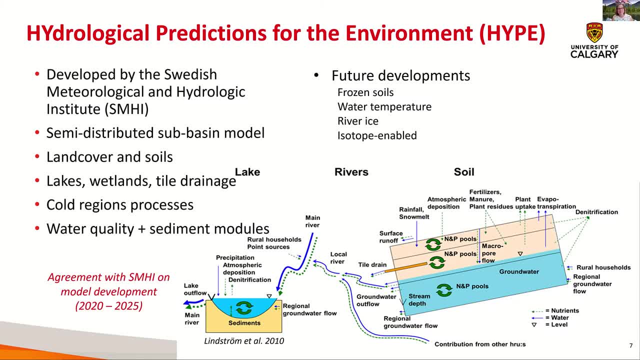 which, when you're looking at millions of square kilometers, is pretty fine resolution. It integrates land cover and soils, very important for Canada. It has a lot of cold regions, processes right from frozen soils to glaciers, And it also has agriculture, so tile drainage, which is really important, as well as lakes and wetlands. 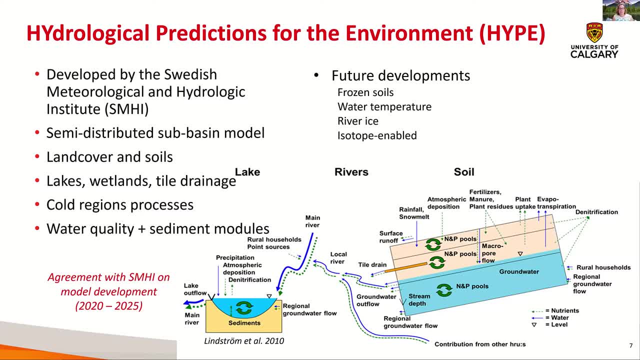 It also has water quality and sediment modules embedded in it, though I personally haven't used those modules. Some developments that my group has been working on: we have an agreement, an open-source agreement- with SMHI and we're helping to contribute to the development. 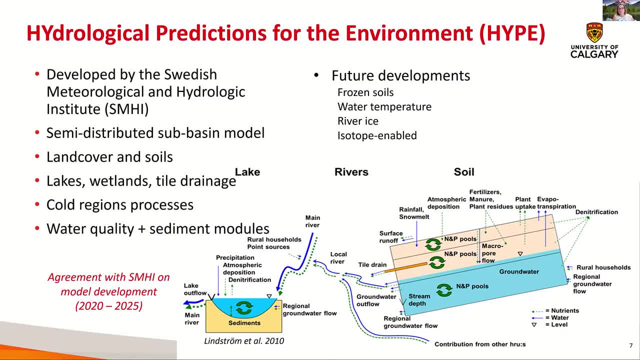 of the model. We've been improving the frozen soils module. We've also worked on regulation, but currently we are working on water temperature and river ice forecasting capabilities and the plan in the future is to actually embed stable water isotopes. We use the isotopes as tracers of hydrological end members or sources. 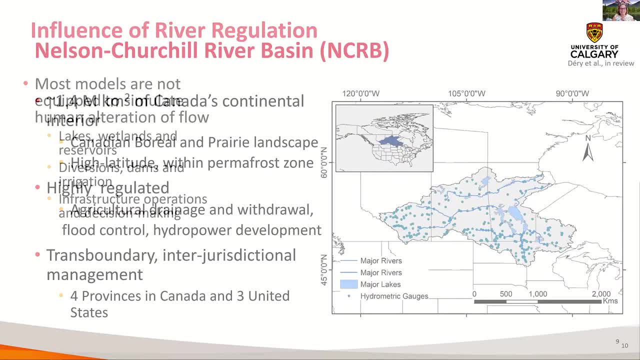 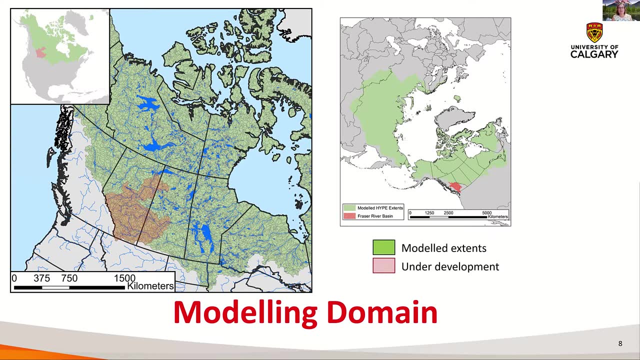 Sorry, there's a lag on my end. The slides are moving forward and not Okay. there we go. So my group has worked with SMHI to set up the model over almost all of Canada now. So that's what the map on the left here shows. 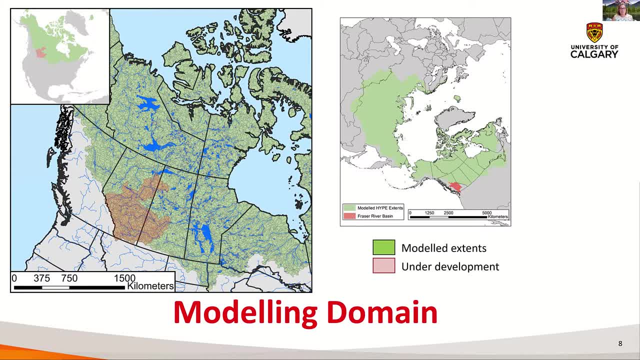 This is from a North America perspective, So we model right from the east coast all the way to the Rocky Mountains. We are now currently working on the Fraser River Basin, which is just to the west here, and we're gradually working our way to the Pacific and the Atlantic. 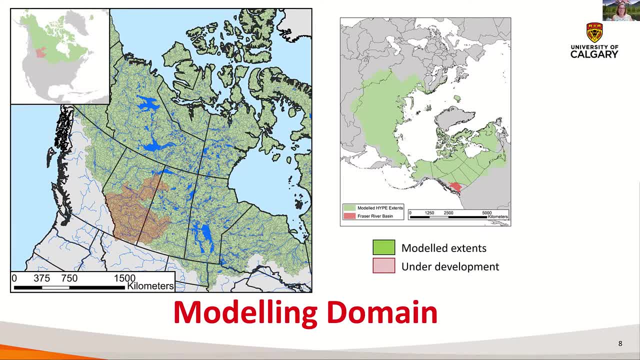 So that just those two pieces that are missing now. After that, we'll be able to provide climate projections for all of Canada, which is important to us in terms of preparing for what's coming and looking at the occurrence of natural disasters. We have also worked on the entire Pan-Arctic domain. 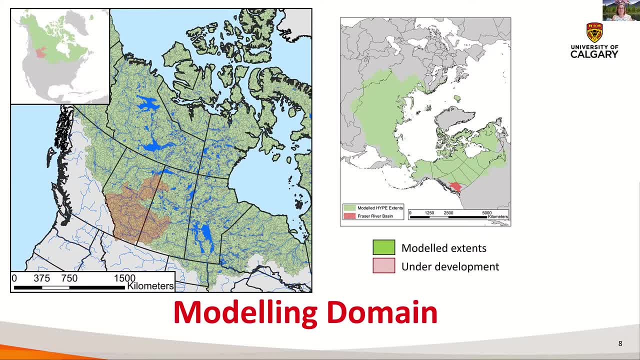 and that's part of my arm of research that is looking at the uncertainty in the Arctic Ocean and how the Arctic Ocean is responding to climate change and how that in turn is driving or fueling more change. So we look at thermal halide circulation and we provide the freshwater runoff scenarios into the ocean for the big ocean modeling teams. 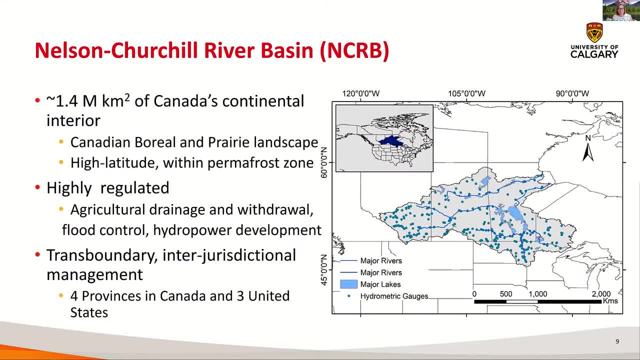 So lots of work going on. The focus of today's presentation and the bulk of the results that I'm going to show you is going to be on the Nelson Churchill River Basin. This is a pretty important basin for Canada because it extends across what we call the Palliser Triangle. 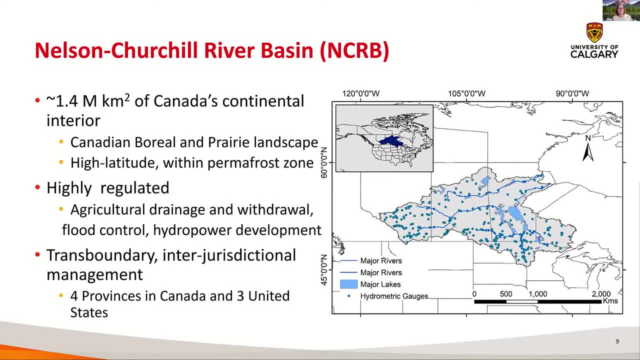 That's a very fancy way of saying something like the Bermuda Triangle right? There's a lot of uncertainty across the prairie region, And so this is Alberta, Saskatchewan, and then Manitoba. This is Lake Manitoba, Lake Winnipeg here, And this is Hudson Bay, which is part of the Arctic Ocean system or drainage system in Canada. 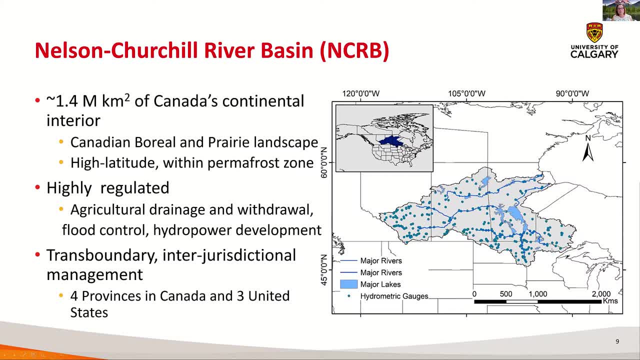 The Nelson Churchill extends down into the US. So this is the Red River Basin and Assiniboine River Basin here And these are the Saskatchewan River Basin headwaters, which is originating at the Athabasca Glacier in the Rocky Mountains. So 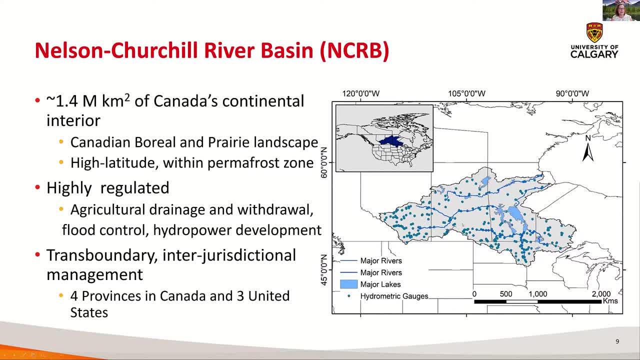 I used to live about here and then I moved over to here, but I'm still in the same watershed, just to put it into context, even though I moved about a 14-hour drive and three provinces over. So significance of this basin. 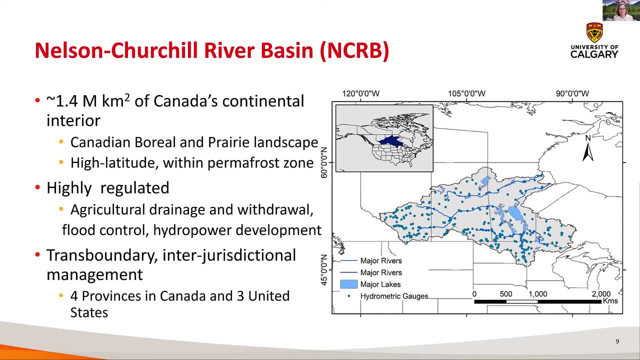 it's 1.4 million square kilometers of Canada's continental interior. It extends across a very important boreal region and prairie landscape, agricultural heart of Canada. High latitude with permafrost within the basin. It's also highly regulated, which you'll see in a moment. 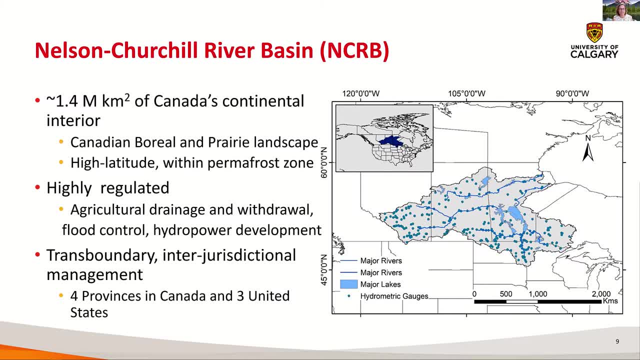 And that includes both agricultural drainage, withdrawals, diversions, flood control, irrigation and hydropower development, And it is also transboundary, inter-jurisdictional, And so we have a governing body here in between Canada and the US called the IJC. 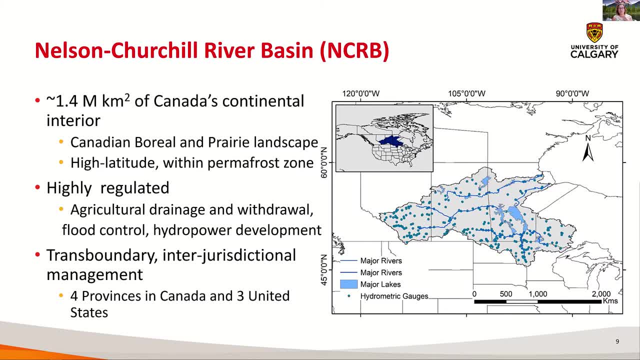 the International Joint Committee, And they regulate how much water is shared across the borders, And so climate change is really calling into question whether the previous agreements that were set about 110 years ago are adequate under today's climates, And so there's a lot of uncertainty to do with that as well. 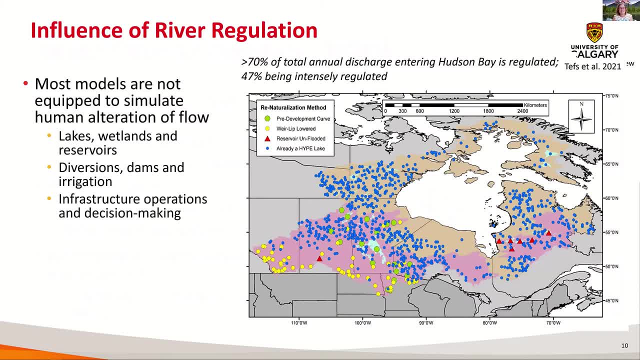 So I mentioned this basin is highly regulated and this is actually showing the whole Hudson Bay drainage basin actually. So all the waters that drain into Hudson Bay, the Nelson Churchill is shown in pink on this end here And you can see that everywhere where there's a dot represents somewhere where humans have altered the natural flow of water. 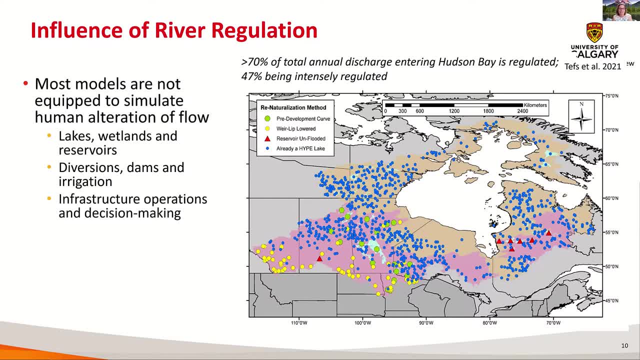 And we've worked over the past three years to incorporate regulation at every single one of these nodes within the model so that we can successfully mimic the amount of water that's making it past those points. And that's really important because the observations- we're calibrating the model to naturally have the regulation recorded in the record. 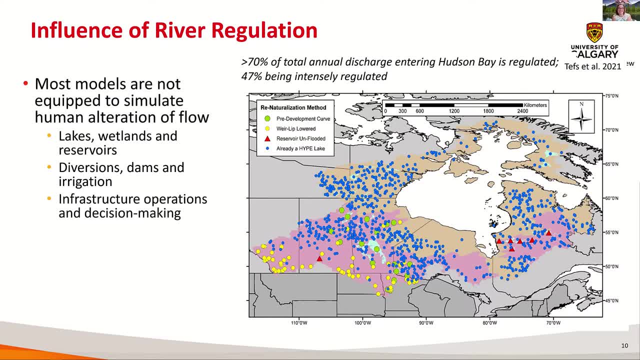 So how can you calibrate a model when it hasn't actually incorporated or accounted for all of these kinds of things? And so some of these points are just simple stage discharge weirs. Some of them are actual withdrawals from irrigation. Some of them are reservoirs where we've had to work with the hydropower industry to figure out how those reservoirs are managed and controlled. 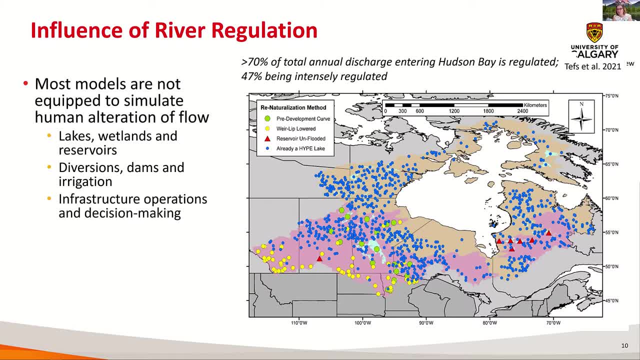 And some of them are lakes, And most of these do not have observed records. So it's been a long three years- Actually, it's been closer to four or five years actually- But I think that it's really important when you're looking at the uncertainty on the landscape of the water and how it's being managed. 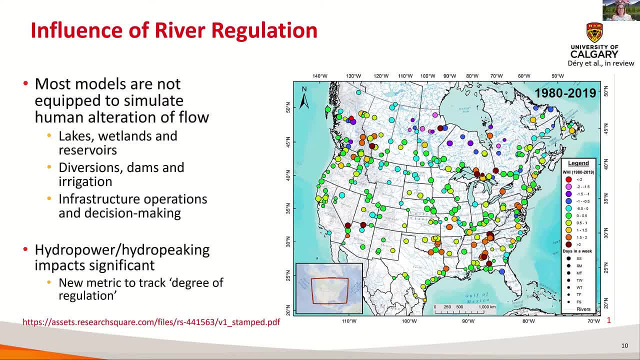 And this is just to show that, in addition to looking at it within the Nelson Churchill River Basin, I've been working with another researcher out of the University of Northern British Columbia and we've extended this approach to all of North America. now I don't know if we're going to go to Europe, because this has been about a 10 year endeavor. 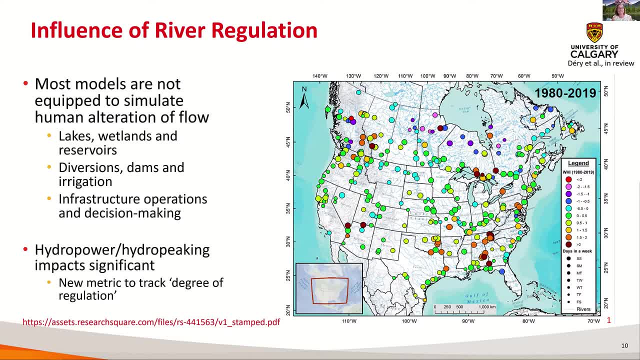 Everywhere there's a point. here is somewhere where we have analyzed the impact of regulation and we've created a new statistical index to monitor the hydro peaking influence in the rivers so that we can actually track the degree of regulation in river systems across North America. 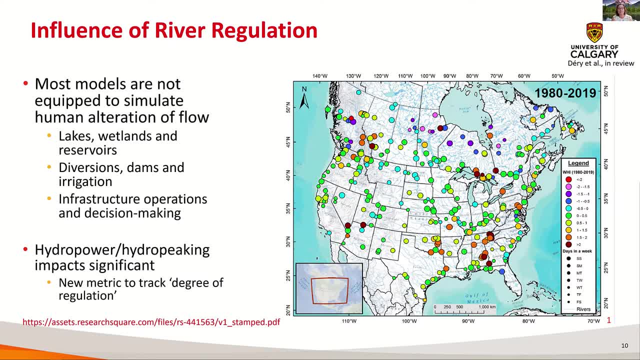 And that paper is shown in red. It's actually posted for comment Right now with nature climate change. So if, if you're willing to provide some input, we would love that- actually anything to help improve the research. So how do we do this? 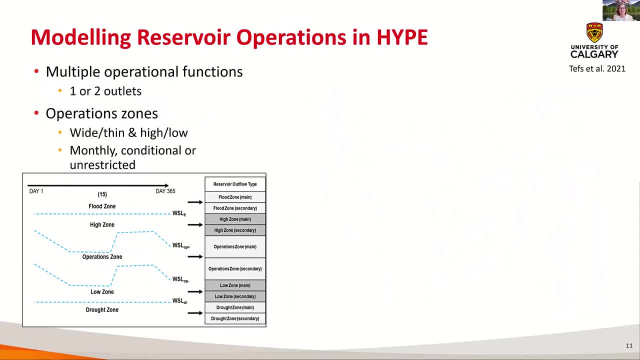 Well, I'm going to present the trickiest part, which is modeling reservoir operations. As I said, we have worked extensively with the hydropower industry in Canada, particularly Western Canada and Quebec. We've looked at multiple operational functions to be embedded. 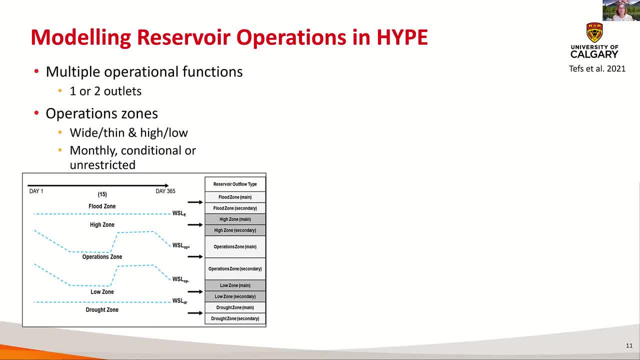 That include reservoirs having multiple outlets, So one or two outlets, because sometimes we get bifurcation reservoirs where the water can actually drain in two separate directions, depending on how flooded the reservoir is, And those are kind of safety measures that are put into place. 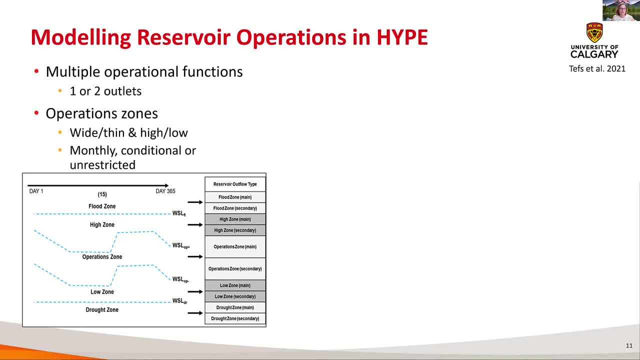 And then we define operation zones within the model. So for every single reservoir there's kind of a target zone, and then there's areas above and below those target zones that have to do with flood zone right here, as well as drought zone. So when you're in drought operations, which they are right now- 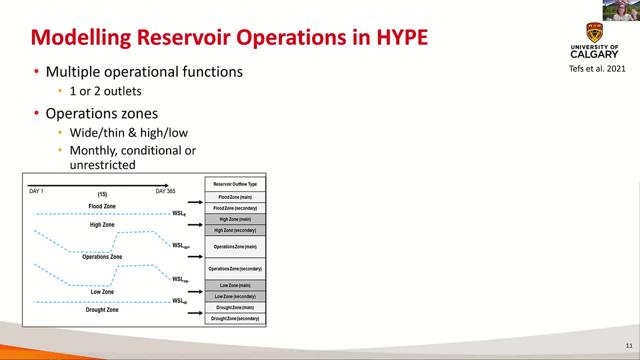 then you have a very different operating procedure than you do when you're in flood mitigation mode, And so that has to do with the way in which we, as humans, make the decisions, and that will then influence how much water is released, And, of course, the goal of this is that we can look at what's happening in the future. 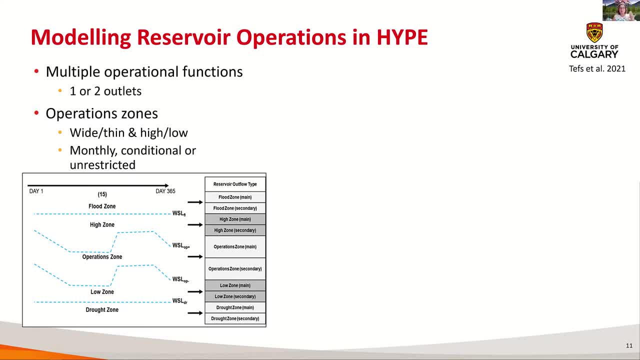 what the impact of those decisions are. And so if there's more frequent flooding, then the reservoir will respond to that, And if there's more frequent drought, the reservoir will respond to that. So that's the advantage of embedding these rules directly in the model. 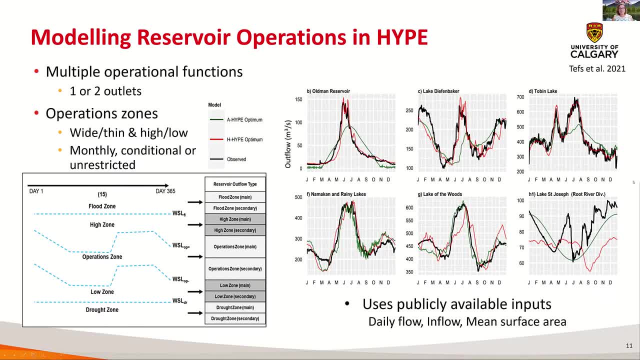 And, as you can see, it has a significant influence on how well the model performs. So this is some key nodes that are regulated with reservoirs within the Nelson Churchill River Basin And you can see the red line or the green line- sorry- represents the model before we embedded the regulation. 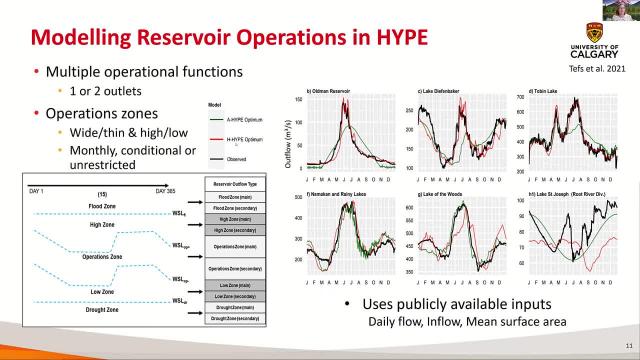 So just the standard height model, And the red one represents the simulated with our operations reservoir operations model and the black is the observed outflow from the reservoir. So I'm not going to say it's perfect. We still have some work to do. 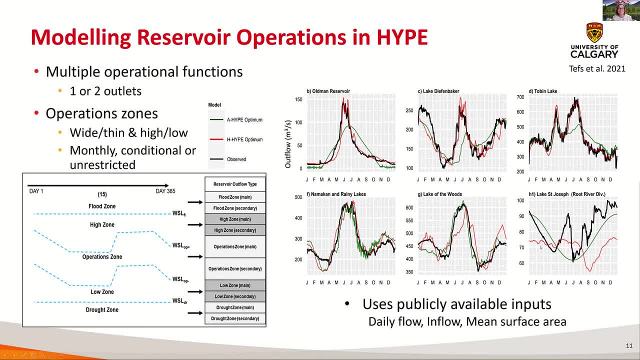 particularly in figuring out some of these more complex systems like Lake St Joseph, which flows from one watershed to the other. It's very tricky to manage, but we're making headway and we're certainly seeing some improvement, And the advantage of this model is that it. 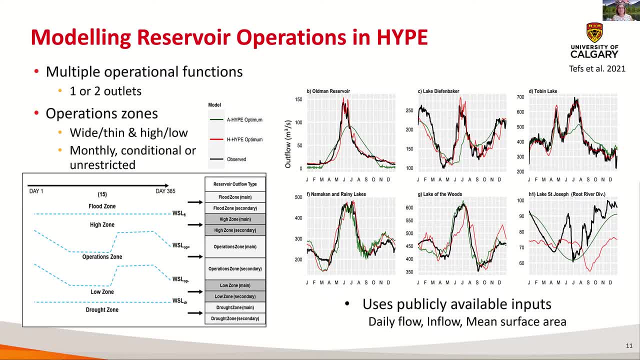 uses only publicly available data and input, So it is accessible for anybody to use, regardless of how remote the location is, And so we're currently working on testing this in Russia right now on some of the large Siberian reservoirs, to actually see how well it performs. 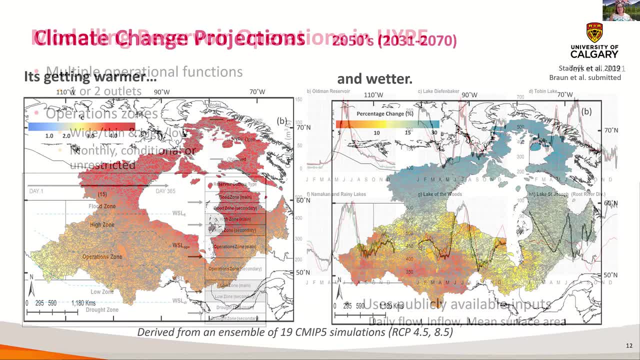 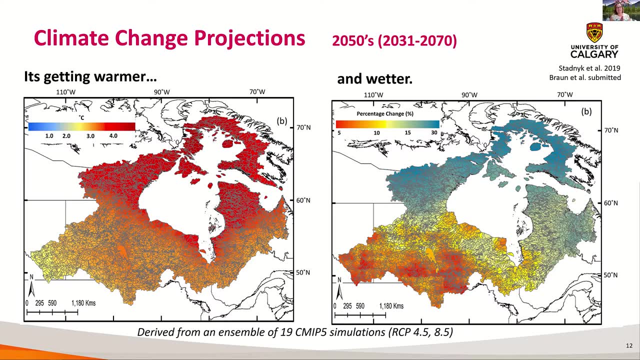 So moving on to the next phase, which is showing you some of the climate change projections and justifying why we're focusing on Western Canada, What we do know is that there's a lot of work that goes behind the scenes. If you want to see the full body of work, 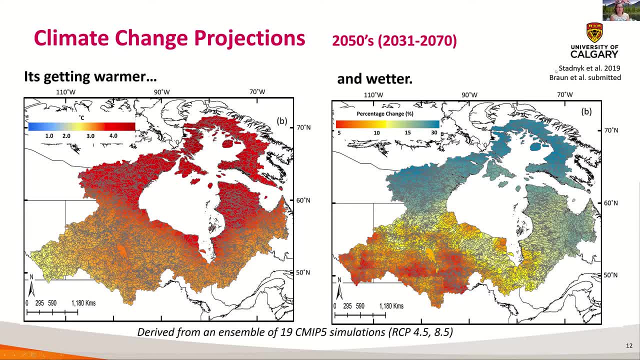 there's one publication that's just been submitted, And then there's also a couple of other publications, the main one being one that I did in 2019.. These are just the projections for the 2050s. We go all the way out to 2100 in some cases. 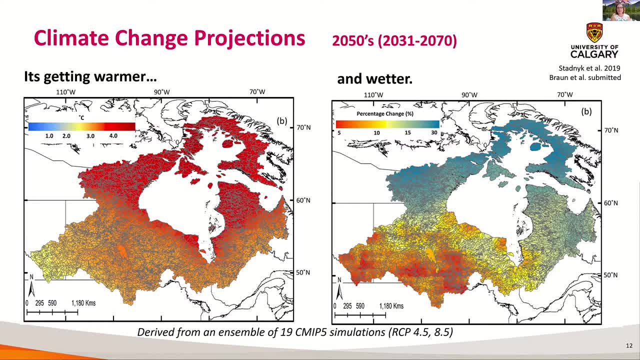 This is an ensemble of 19 climate models that was fed through an ensemble of hydrologic models, And what we do know, or one thing they agree on, is it is getting warmer. It's just a question of how much warmer And, generally speaking, things are getting wetter. 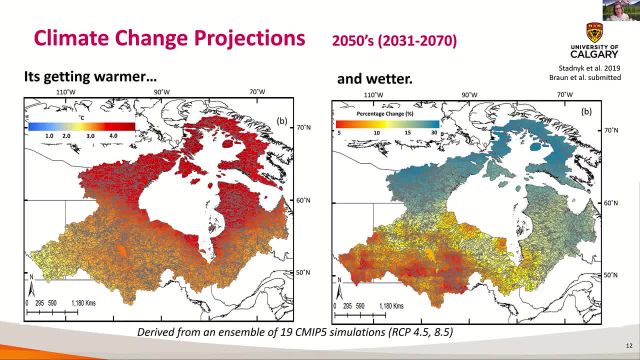 There's a huge discrepancy, though, in terms of how much wetter, depending on where you are, So what you can see from the panel on the right here is, if you're anywhere in Northern Canada, it's definitely getting a lot wetter. 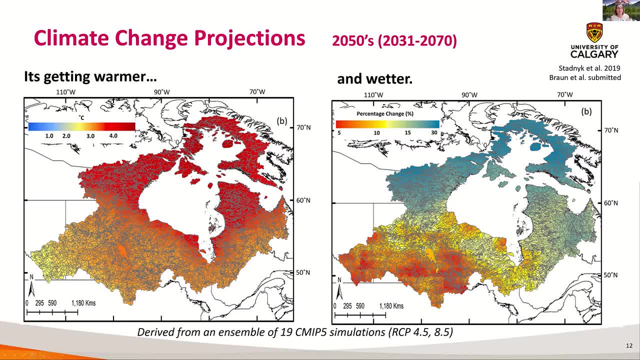 And that largely has to do with the fact that the atmosphere is a lot warmer and the seasonality is changing. But if you're over the prairies, this tricky little region that I was talking about, the Palliser Triangle- it is getting wetter, but only by about 5% on average over long periods of time. 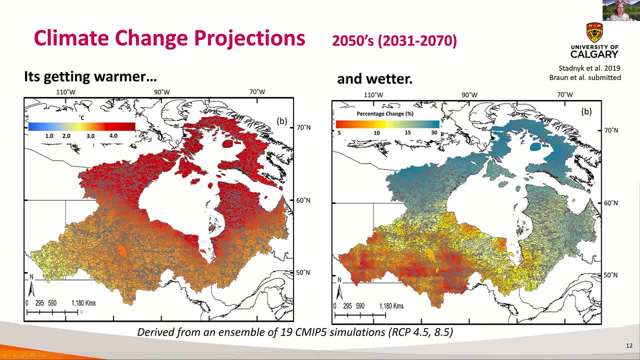 And so that raises a few questions, because it's certainly getting a lot warmer, but only a little bit wetter, And so when we look at the non-linearity that I talked about at the beginning with hydrology, that has a significant impact in terms of the amount of runoff. 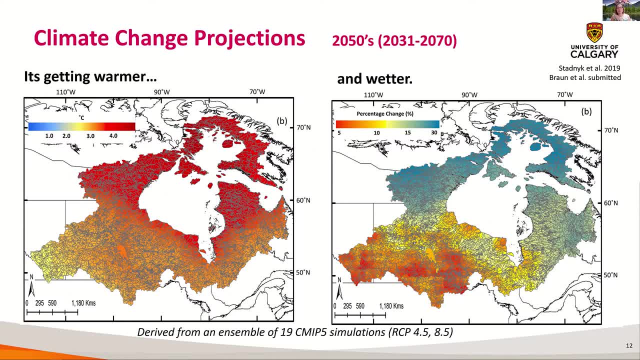 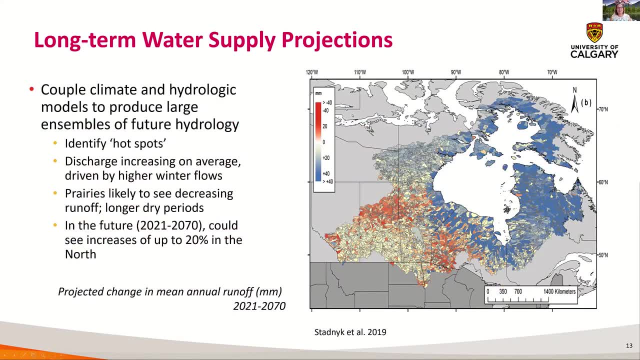 So what we can see here is, when you combine just a little bit wetter with a lot warmer, you actually end up with the scenario where runoff can actually be decreasing, And the main reason for that is hot spots where evapotranspiration is throttling up that much more. 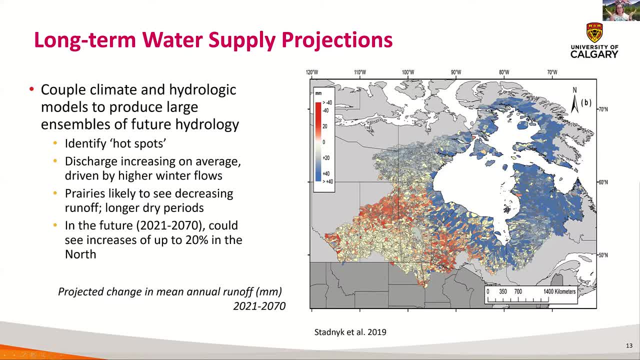 So a little bit more moisture, a lot warmer, you increase evapotranspiration And over regions that are already inflow limited or already have issues with the amount of water availability and are already naturally dry, that creates a multitude of uncertainty And you can kind of see that represented. 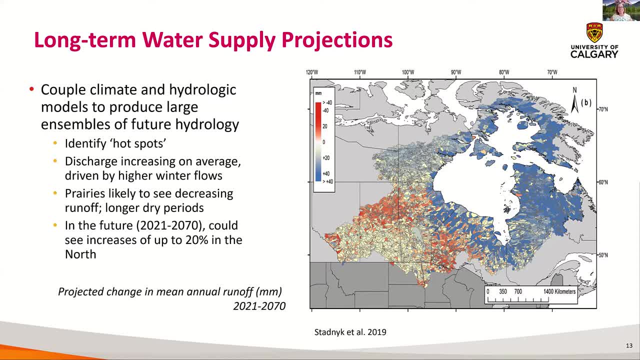 by this piecemeal diagram here, where clearly things are getting wetter more runoff on the eastern side of Hudson Bay but on the western side there's a lot of discrepancy And for sure it's getting wetter in the north. 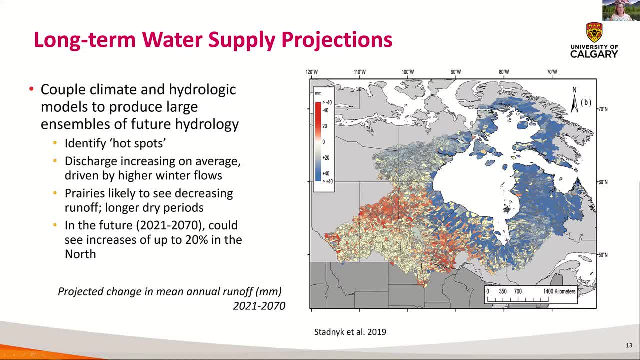 but this kind of zone of uncertainty extends fairly far north. It is getting wetter up here for sure. Down here we don't actually know if it's getting wetter or drier, and that presents some considerable challenges for managing water On the landscape. 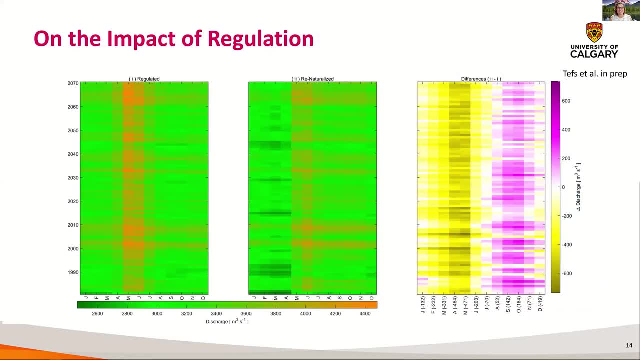 And if you recall from my regulation diagram, it was also the area that is very intensely regulated. So what does that mean for any kind of water resource operator or practitioner? Well, we definitely need to consider the impact of our regulation decisions And with this diagram here it's pretty complex, but I'll break it down for you. 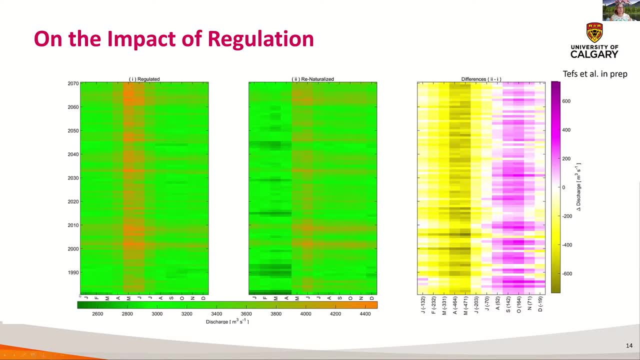 On the y-axis is your time series, So going from 1981 all the way up to 2070.. On the x-axis represents the different months of the year, So we've broken it down into monthly blocks and the colors represent the amount of discharge. 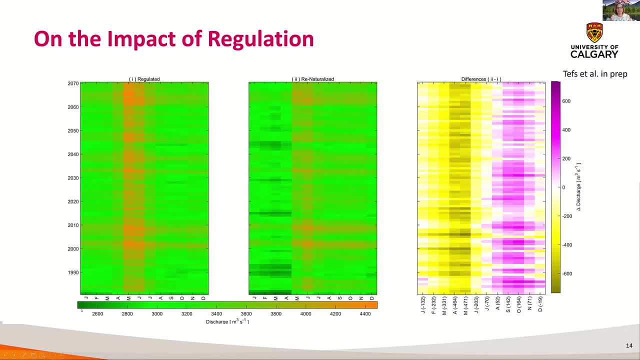 So the orange is higher and the green is less. So you can certainly see the peak flow happening here, And what you can see when we have a regulated model is that there's a more exaggerated peak flow season and then the shoulder seasons that it drops off. 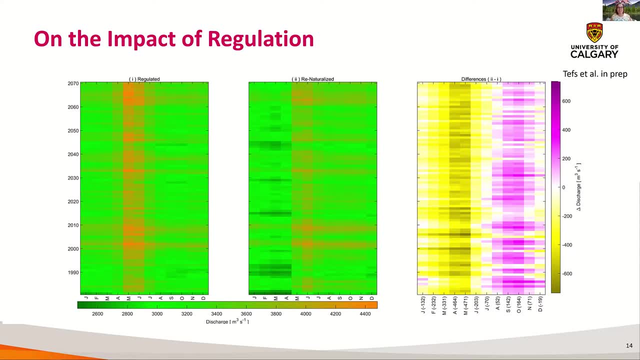 So, if you picture your natural average annual hydrographic shape. when we re-naturalize the model, though, and what this means is taking the regulation rules out of the model and rolling back the land cover, as if those reservoirs never existed, or those withdrawals and irrigation tile drainage never existed. 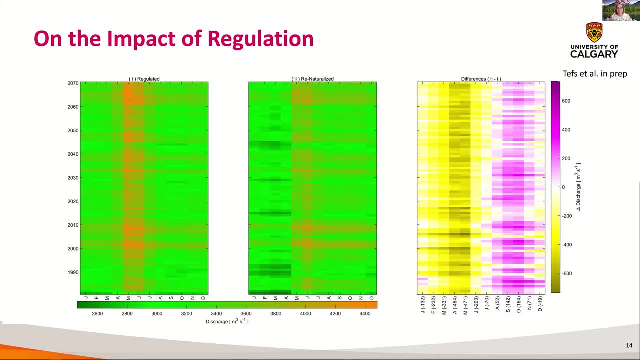 You take all of that out of the model and we run it in today's day as well as the future climate, as if regulation had never been built in the watershed, And what we see is a much more piecemeal, a lot less consistent, but a much more consistent model of regulation as well. 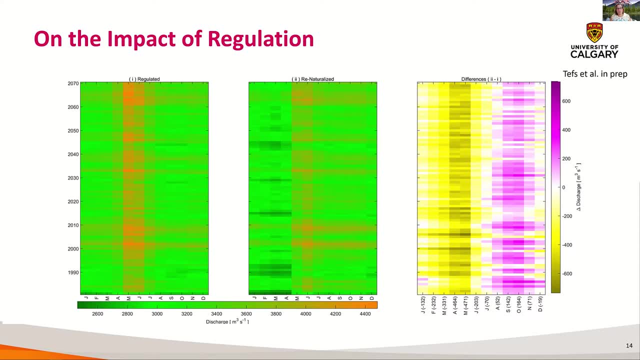 And what we see is a much more piecemeal, a lot less consistent, but a much more consistent model of regulation as well. consistency to the hydrologic cycle and the way in which it responds to climate, And so the moral of this story is that regulation has a significant impact, but not necessarily where you'd expect to. 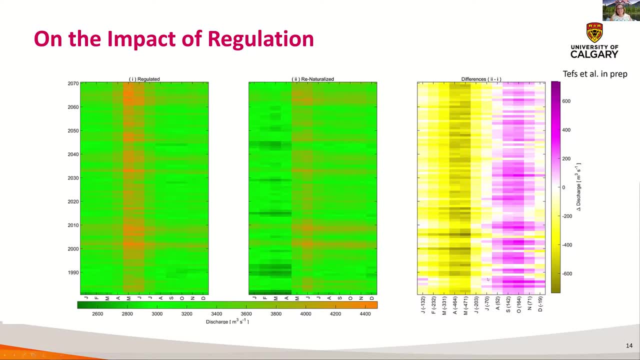 see it, It's actually the peak flow season that's the least impacted. The majority of the impact occurs on the shoulder seasons, So during those fall, late fall and winter flows, which is where you have these critical low flow periods or ecological flow needs. So those are the periods. 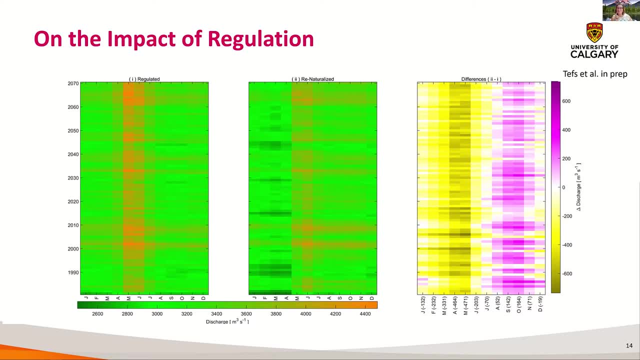 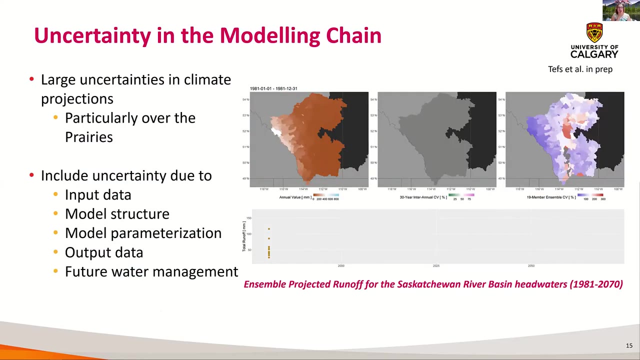 of time that we actually have the most uncertainty, And that's kind of contrary to what we think as hydrologists. we may think of it from a flood forecasting point of view. So for climate change it's those shoulder seasons that matter the most. All right, so dealing with uncertainty in the 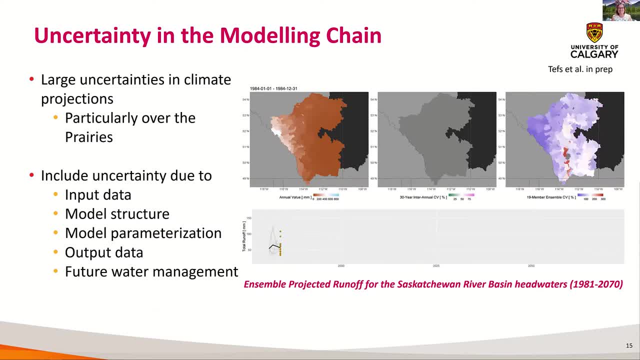 modeling chain. I think I've presented that there's quite a bit of uncertainty that we need to be aware of. There's certainly large uncertainties in the climate projections, particularly over the prairies. This is showing the headwaters of the Nelson Churchill, the Saskatchewan river basins. 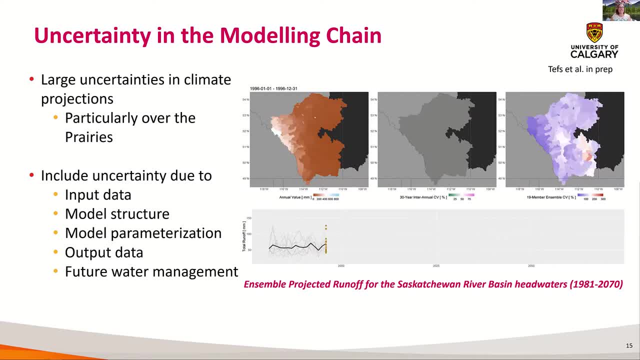 the North Saskatchewan and the South Saskatchewan, And this is a time series animation of the average annual runoff, as well as the 19 member ensemble in terms of the coefficient of variability. And down here is the time series of runoff showing how, if we take the different seed values, that 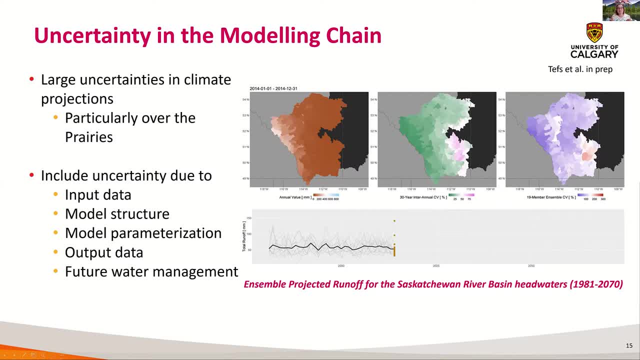 account for the different uncertainties. typically speaking, we report only the mean, but you can see the spread is actually quite high And if you're an operations person, that becomes pretty tricky to deal with. And that's what we're really focused on is how to help operations make sense of this. 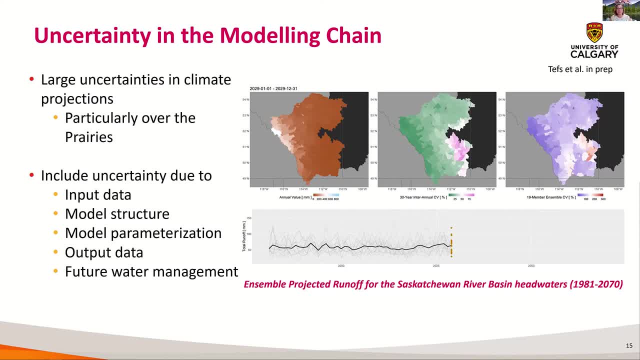 but still account for it because we maintain that we need to do that to better understand the risk. So we look at things from input data uncertainty to the model structure or model choice, model parameterization, output uncertainty. There's uncertainty in our observations, particularly. 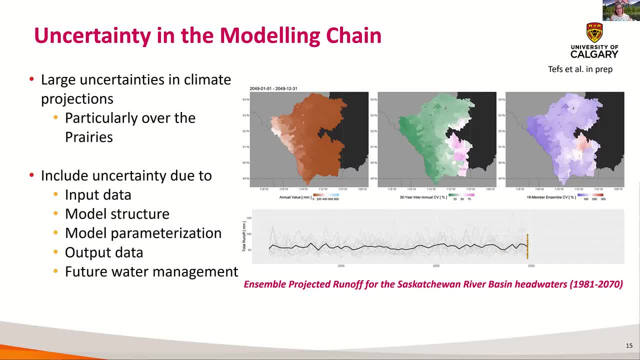 in Canada, because of ice on versus ice off, We can have up to 80% uncertainty for ice affected ratings, hydrometric measurements. So that's pretty significant when you take that into account, as well as the regulation and the future water management. 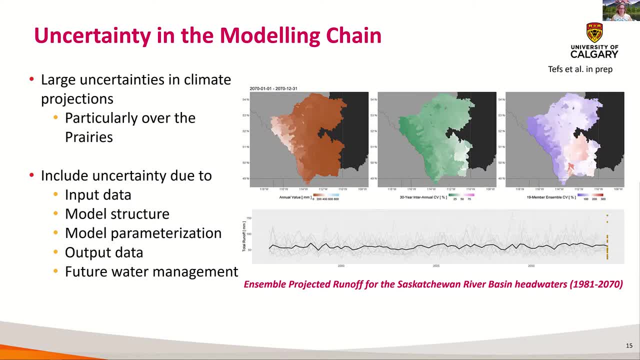 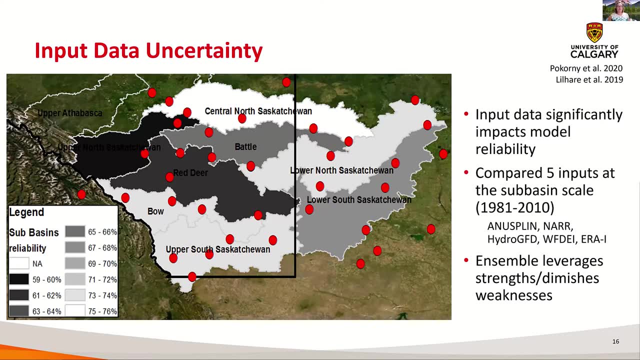 Okay, Sorry, this slide is Slow. There we go. Okay, So taking a look at input data uncertainty, this is just a sample again, but we have worked to compare different types of historical data that drive the model. This is showing the comparison of those different products. This was an ensemble of five different. 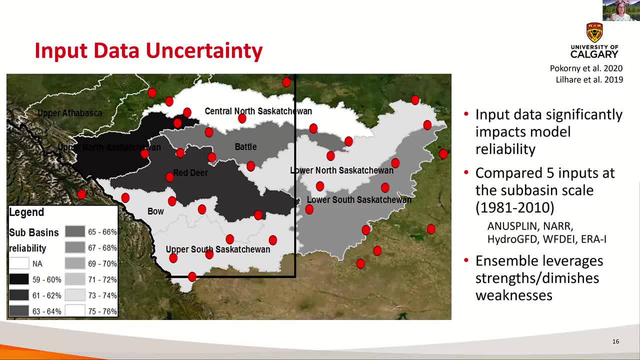 inputs at subbasins across the Saskatchewan River Basin from 1981 to 2010.. And we basically looked at the reliability of the data. And we looked at the reliability of the data And we looked at the variability in terms of the agreement in the model output as a result of changing only the 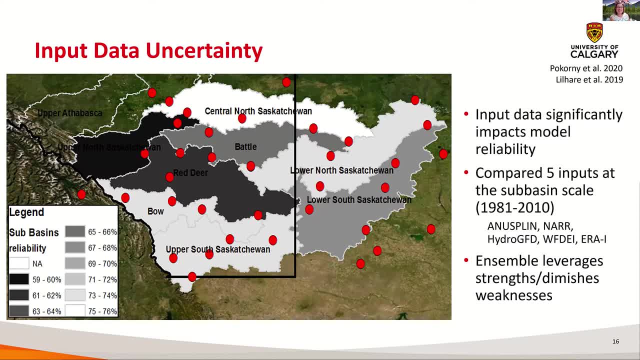 input data, And what you can see here is the spread simply from changing the reanalysis product. And all of these reanalysis products are considered to be used in operations or are currently used in operations in Canada, So they're very reliable products, but there's huge discrepancies, even in terms of what we think we know about the historical climate. 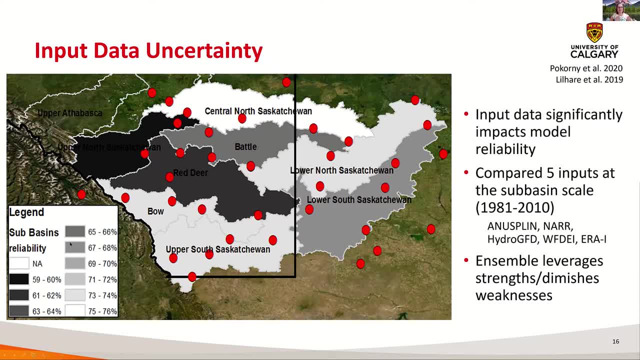 So we would then feed that into the hydrologic model and produce an ensemble of outputs that's based solely on varying the inputs. But of course, that's only one source of uncertainty. We also have to consider output data uncertainty, And this map shows you. 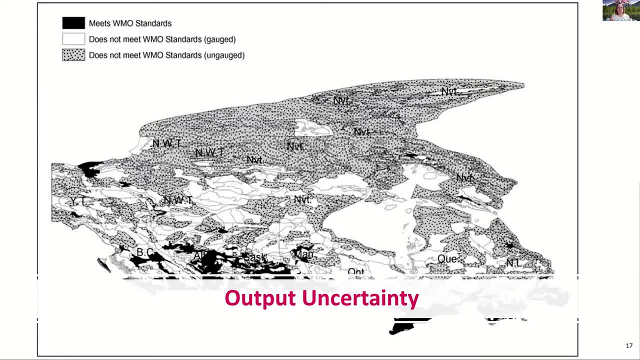 the challenge that we face in Canada. This is from a review done back in 2013,, and it shows the percentage of basins within Canada's hydrometric network that meet WMO standards for being reliable in terms of having adequate hydrometric observations, And what you can. 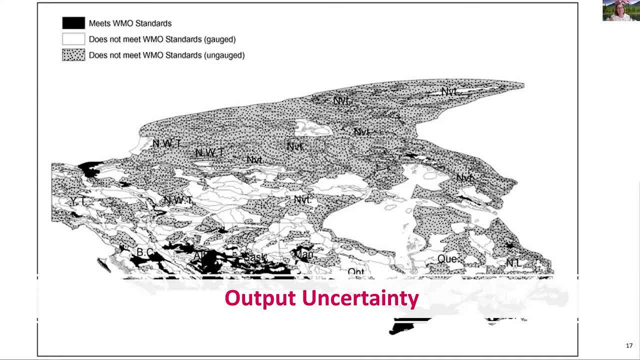 see is that the majority of Canada does not meet is either ungauged or undergauged. we don't meet the World Meteorological Organization standards. In fact, greater than 80 percent of Canada's terrestrial landmass does not meet the World Meteorological Organization standards. The places 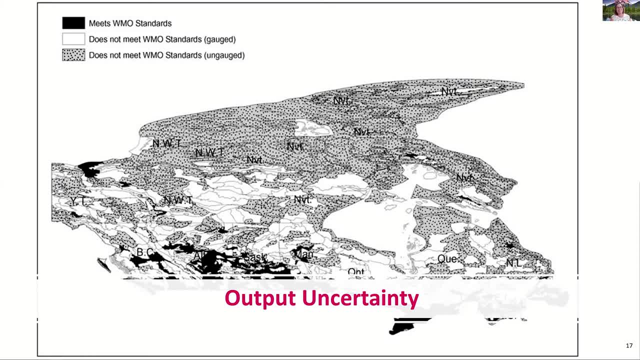 that do are, of course, focused in the south, along the Canada-US border, because of the transboundary waters, also because of where the population resides. So there's a need for more hydrologic data, And this doesn't even get at the whole issue or discrepancy between frozen and unfrozen. 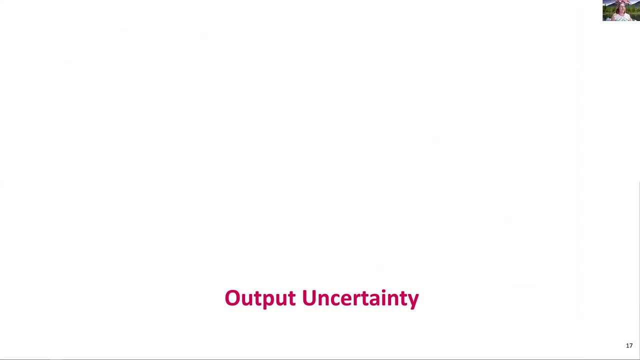 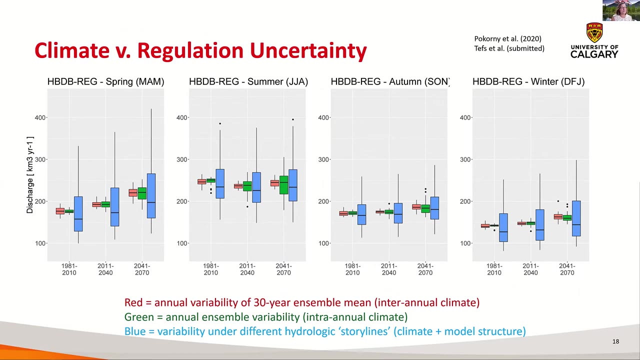 rating curves. Then we also have uncertainty that's added because of human decision making and regulation. And what this series of plots is actually showing you is what happens when we compound uncertainty. So we take the input. uncertainty, that's looking at the red boxes in these box whiskers here, So simply looking at the variation. 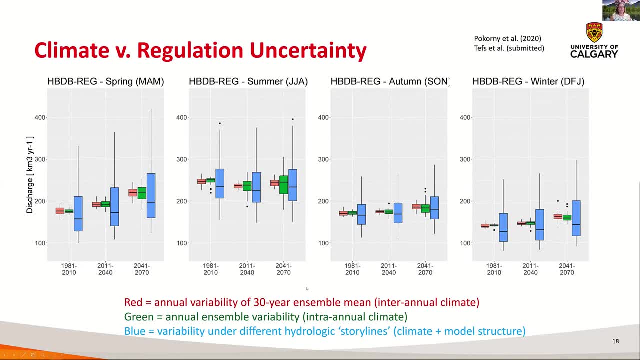 of inter-annual climate, then you get the red box. If you look at the green, then with the green we are varying the model structure, So regulated versus not regulated, And so we're adding that uncertainty together And with the blue that's the incorporation of all uncertainties, the input: 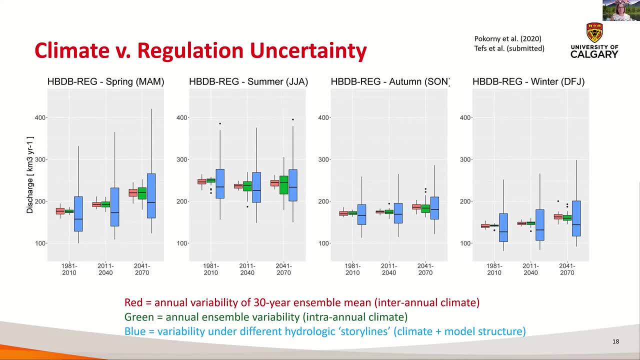 the output, the regulation making on the landscape, as well as the climate change uncertainty, And you can see the compounding effect here. It's probably not a big surprise, But of course we treat that differently And when we report our model observations or simulations we have to be mindful of this, And I'll talk about 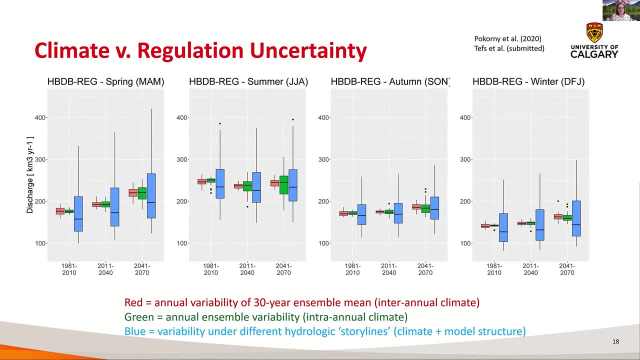 that in a few minutes. But the other thing I want to say is this also affects how my team calibrates our models. If we know that our target is the blue box, we're not going to worry about a NASH score one or trying to get above 0.9.. Because we know that the best we can possibly aim for would be. 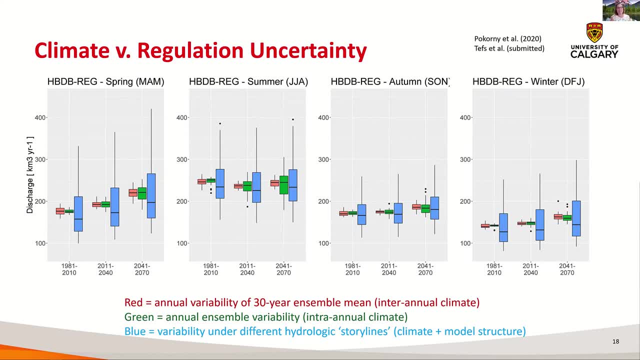 say 0.75.. And everything after that is meaningless. That's important because then we're not overtuning the model And we're allowing the model to be more flexible and less rigid on a continental scale. So the question is, does this matter? And I wanted 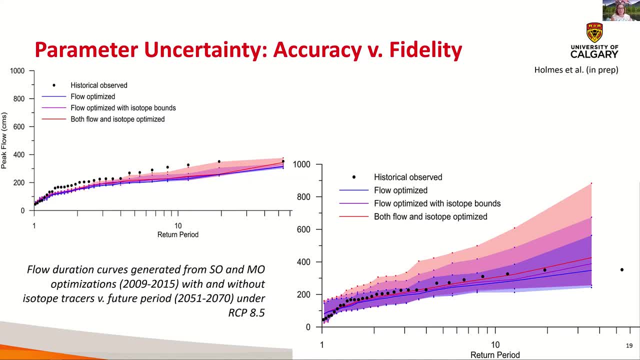 to show you this. This is actually from some of our isotope simulation work, where we're really checking processes and making sure we put the water in the right place And we're going to put the water in the right bucket on the landscape, But this shows you the impact that that has. So 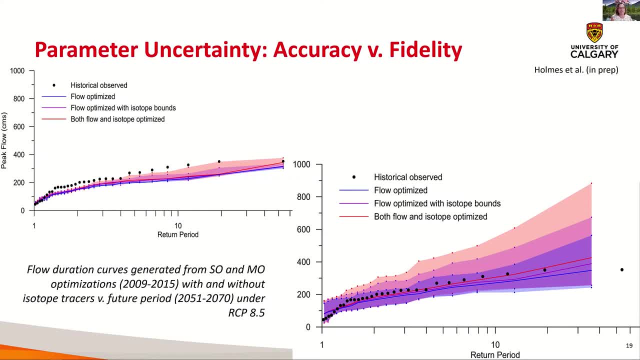 all of these simulations that were done, that are shown here by the ranges and by the dots, which represent the mean of each of the range for the different colors, were all NASH scores above 0.8.. So they were statistically the same in terms of overall stream flow, But there was huge. 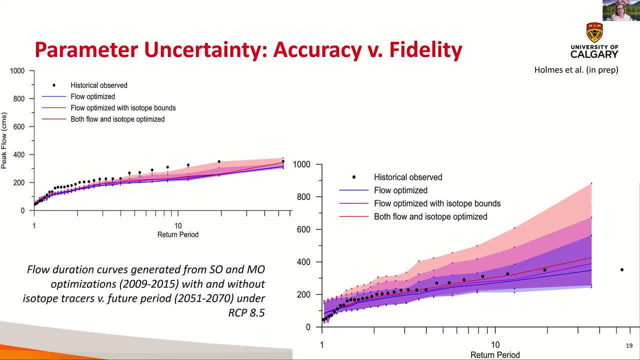 variances in terms of where the water ended up on the landscape, in terms of what the buckets and what processes, And you can see that for the historic flow duration curves on the left-hand side here there wasn't really a significant difference in terms of how we 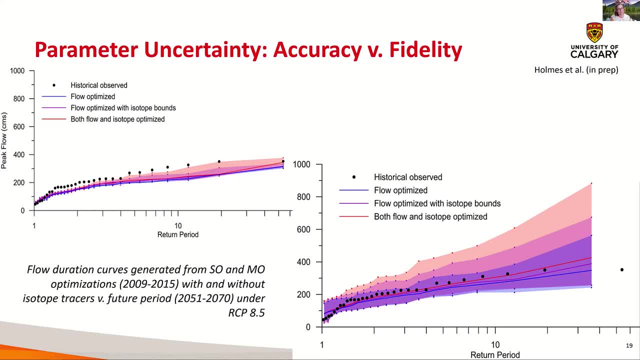 parameterized the model, But when we drove that model into the future, then all of a sudden, particularly for the high flows or the higher return periods, there is a significant difference in terms of where that water ended up and what flow you end up with. I don't know about you. 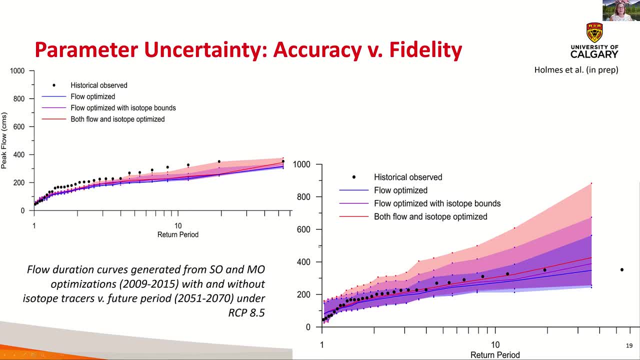 but if I'm managing a reservoir, I'm going to have a lot of flow, And if I'm managing a reservoir, knowing that my max flow for the future is 500 versus almost a thousand, that's a pretty big operating range And I think that it's very important for us to consider not just overall. 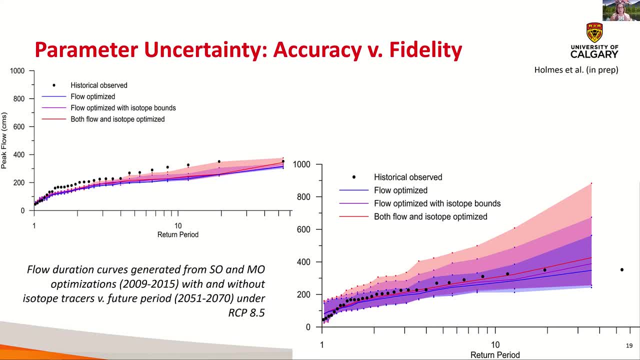 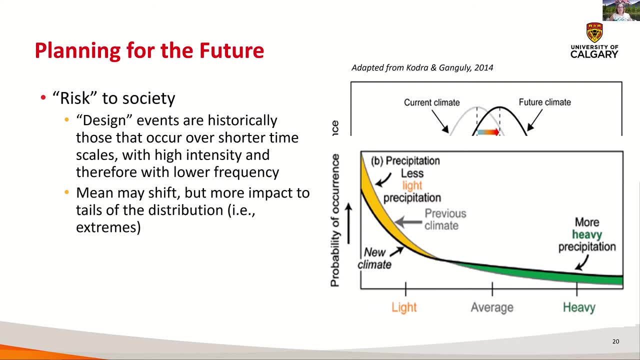 stream flow simulation accuracy, but where we're putting the water within the model. That's also very important. So, in terms of how this impacts operations and how operations can deal with this, I wanted to show this for the students just to highlight that the true risk for society is that when we in engineering coin a design event, 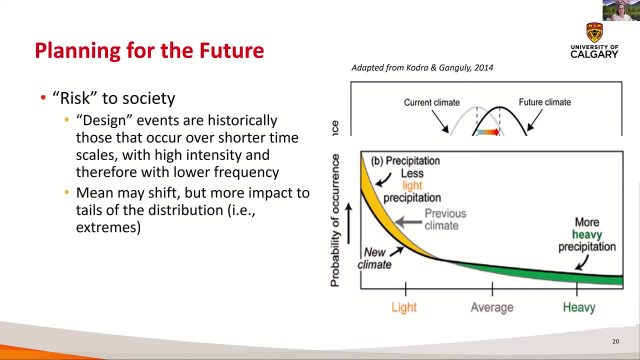 historically, those are the events that occur over shorter timescales with higher intensity. That's when we were talking about IDF curves. that's really what we're looking at And this may mean a shift, but it's, generally speaking, not a shift to the mean, And you can. 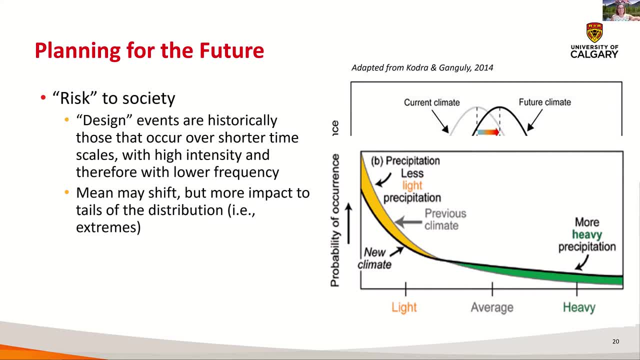 see that here represented. sorry, I can see the animations kind of screwed up, but that's fine. We can talk about it from the duration curve. It's not a change in the mean. That's where the two simulations kind of cross over. but where we're really impacting things is on the tails of the distribution, the least common. 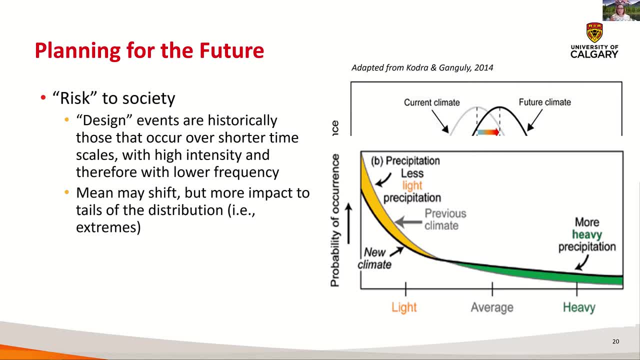 events that don't occur very often And those are also, ironically, the events that we have the least amount of data on, because they don't occur very often in the case of drought And in the case of flood, typically those events wash out our gauges, So we don't have really a good handle on what a 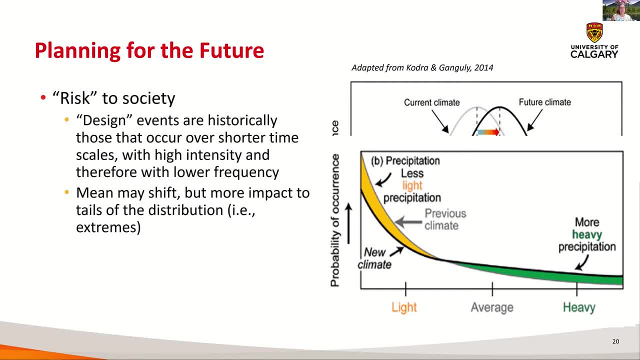 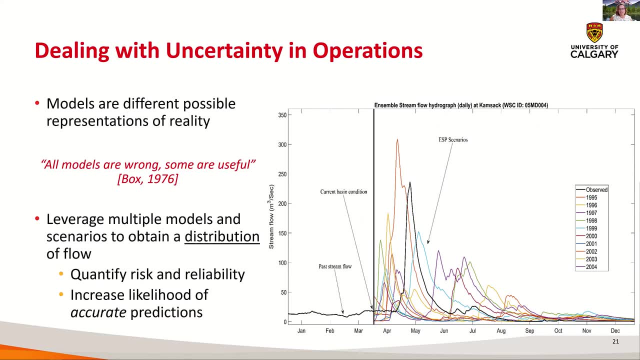 500 year flood is Okay. So when we talk about dealing with this uncertainty in operations, our team will aim to produce the uncertainty envelopes for operational decision makers. They don't often have the time to set up multiple inputs for the same hydrologic. 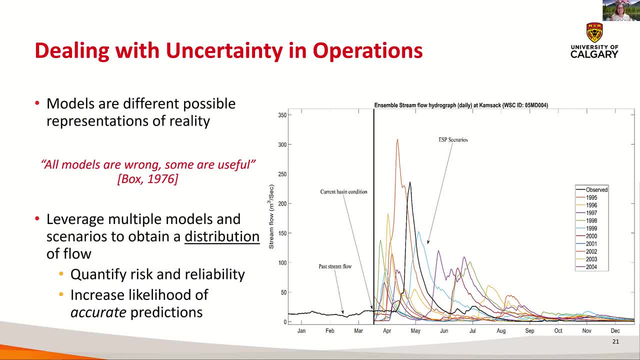 model or different parameterizations and explore all of that uncertainty. We would hand that over along with a tool that will help them to define risk-based scenarios from those distributions. So we think of it. if you take a time slice so you pick any month. 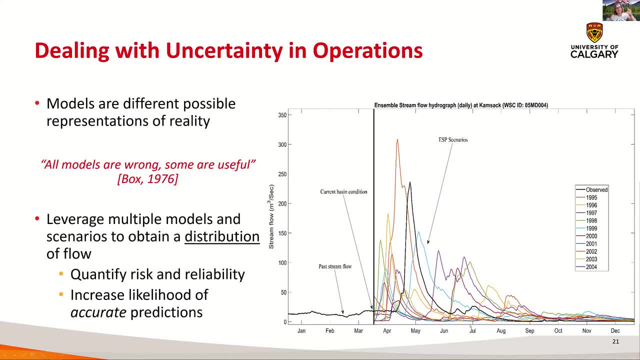 let's say July, and you cut through here if you turn your head sideways. you can create a probability distribution function from that, Because of the fact that there's going to be some that are on the tails- least likely or most extreme, either low or high. 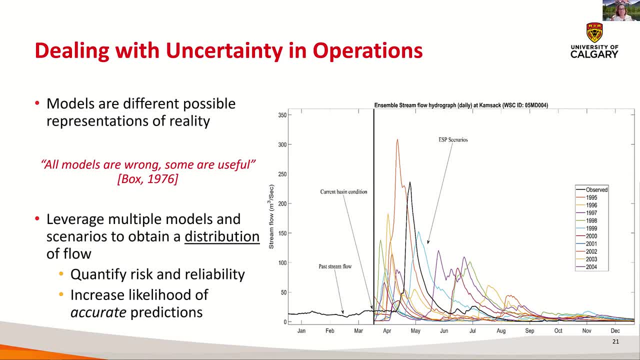 and those that are more common, which we know to be the expected value or the mean. So for every point in the hydrograph in time, we'll create a probability distribution function that can then be turned into a cumulative distribution function that allows the operators to take a risk-based 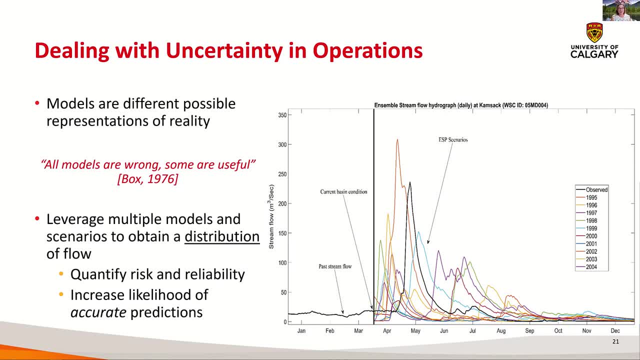 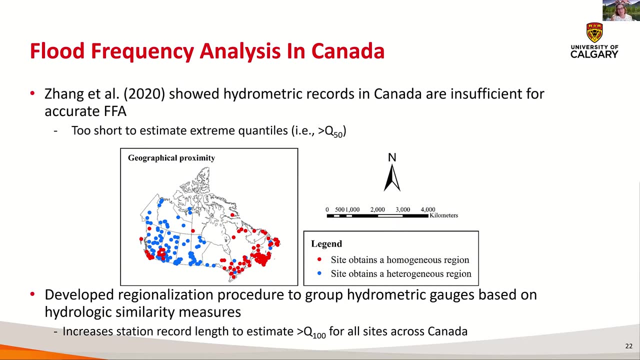 approach to decision making, So they don't have to decide on their own which scenario is most likely. They can actually look at it in a slice of time or at a certain point of time where they're most interested. So doing this presents its own challenges. For one, if we talk about flood, 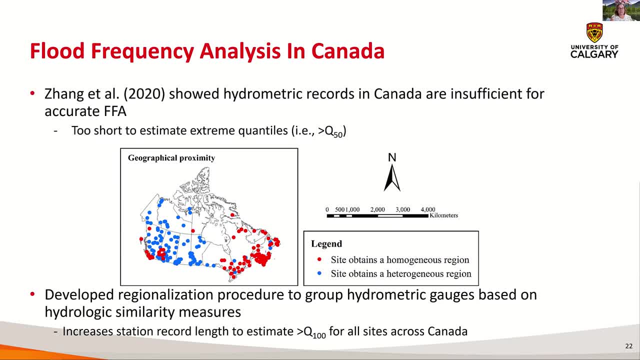 frequency analysis in Canada. I already mentioned that our hydrometric network is generally inadequate to produce the design events that are of interest Most of our large water operating infrastructure. it has a design life of 100 to 500 years And our longest record in Canada is about. 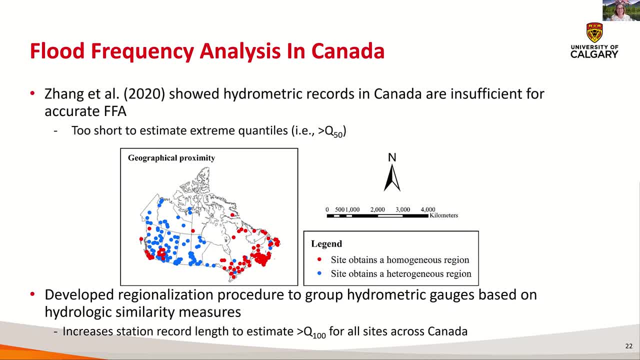 110 years old. Actually it might be closer to 130. But anyway it's not very long And generally the rule of thumb for doing any kind of flood frequency analysis is you need two times the return period. So if you're interested in a 500-year flood, you need 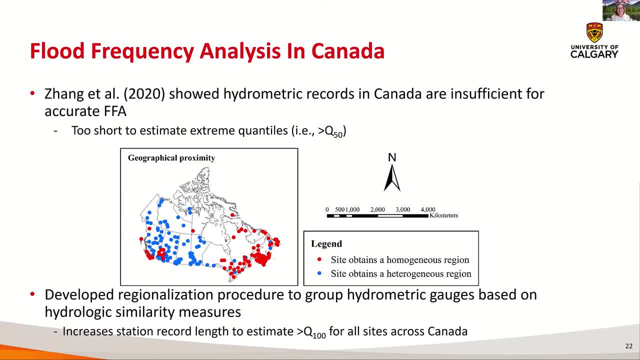 1,000 years of data. We don't have that Surprise surprise And there's lots of uncertainty in the model simulations. So one of the things that my group has worked to do is to develop regionalization procedures where we can determine which gauges belong to a like group in terms of 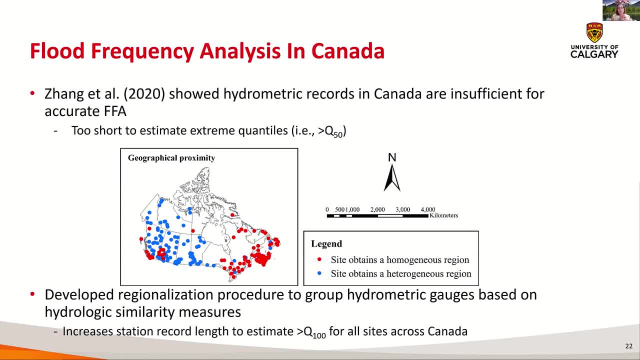 how they respond hydrologically And we can pool those records to actually extend the period of time, And we've managed to successfully do this for all regions of Canada for greater than a 100-year design life And we're working on extending that even past a 100-year design life. 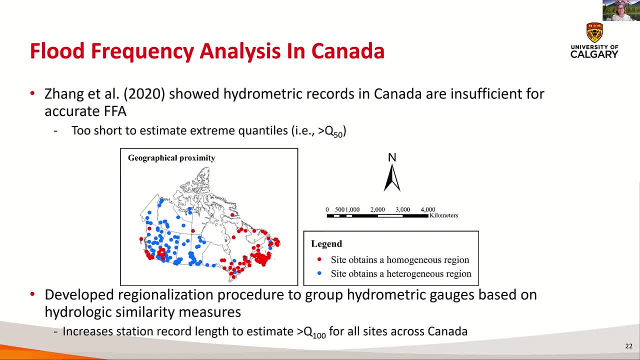 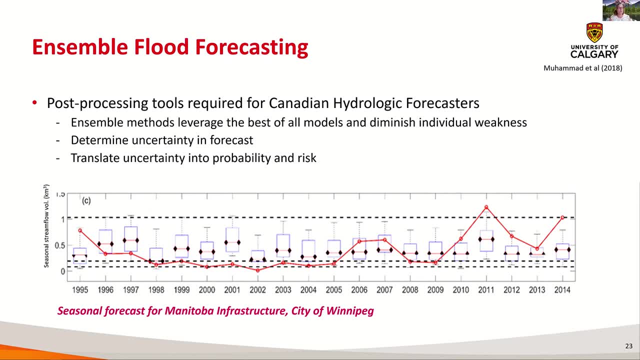 So we're helping to create data to compare to for these design events. We've also created ensembles. This particular one was for the city of Winnipeg, for Manitoba infrastructure, where we set up multiple models, multiple hydrologic models, and modeled some significant events in history. 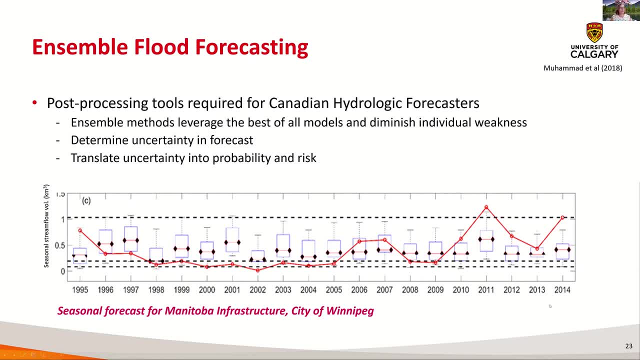 We did do a historic record. We've also done a future record. This was seasonal forecasting, So predicting flow on a seasonal or a monthly basis and plotting them as box whisker plots so they can actually interpret each slice in time on a monthly scale. I'm showing it here: 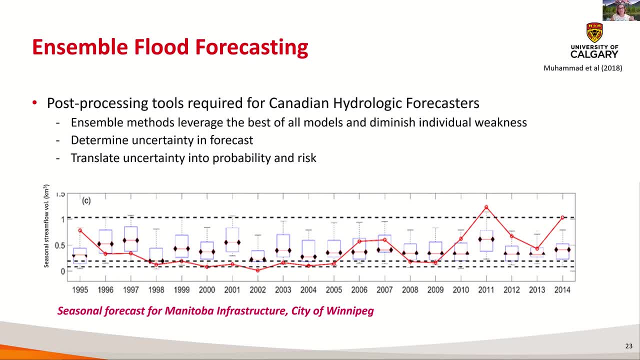 annually as a risk. So 25% probability, 50% probability, 75% probability And the red shows the observations. And even for the significant event in 2011, we did pretty well. Granted, it was up on the upper tail, but you would also expect. 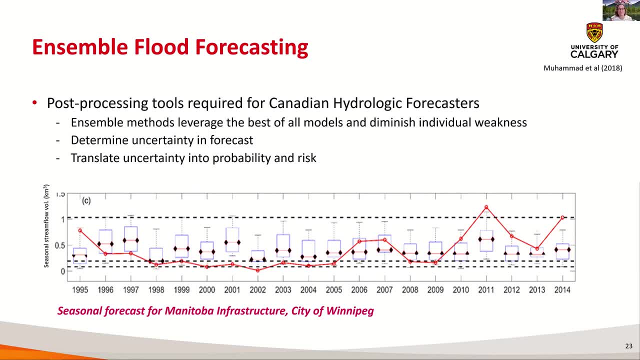 it to be on an upper tail, given it was a 1 in 250 year flood at the end of the day. So see that there's a chat. Okay, perfect, I'm almost done anyway, And so I also wanted to address what 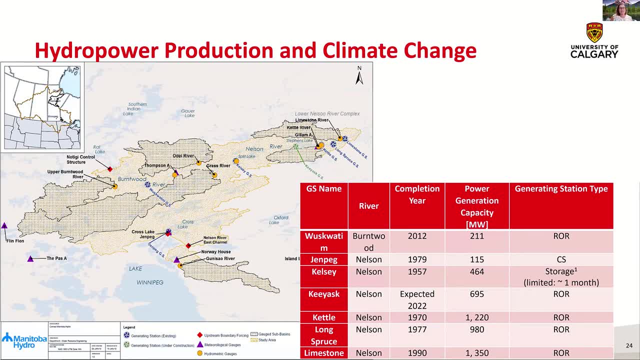 we're doing for hydropower industry. We've done a lot of work within the Nelson Churchill, particularly with Manitoba Hydro. We've also worked with Quebec. This is showing some of their major hydroelectric generating stations, So you can see in blue. 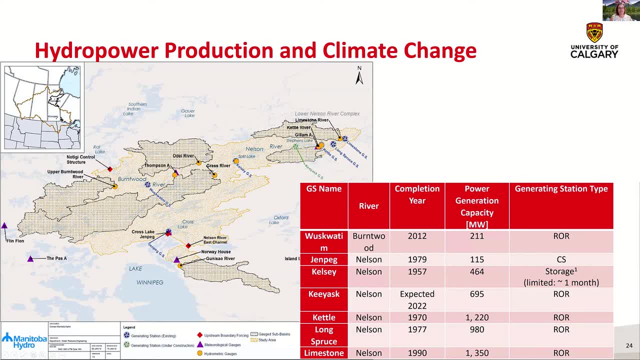 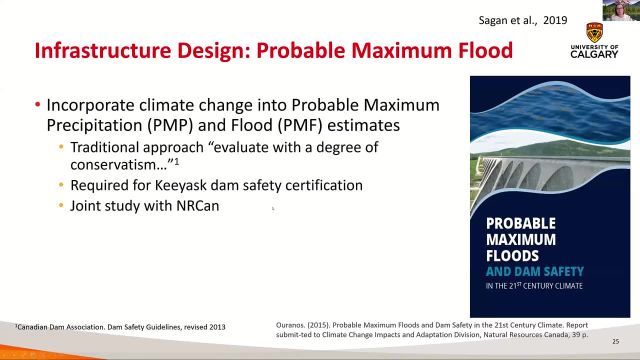 as well as in orange. those are all control points within their system. The work that we did here was to look at probability, probable maximum flood in response to probable maximum precipitation. The biggest problem in Canada is that we Engineers. Canada has released a statement. 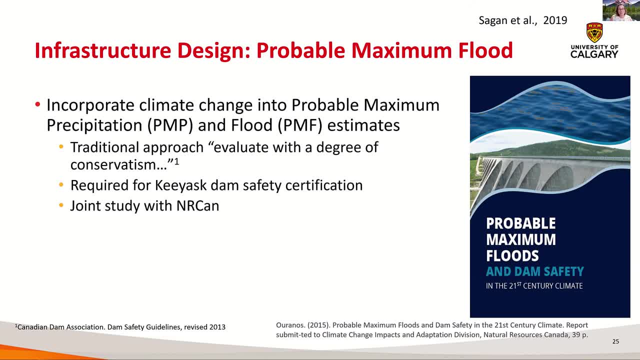 saying that we need to account for climate change, but there isn't a set procedure to do so, So operations and utilities have a hard time knowing how to incorporate climate change. So we did this in response to a dam safety certification that was happening for a brand. 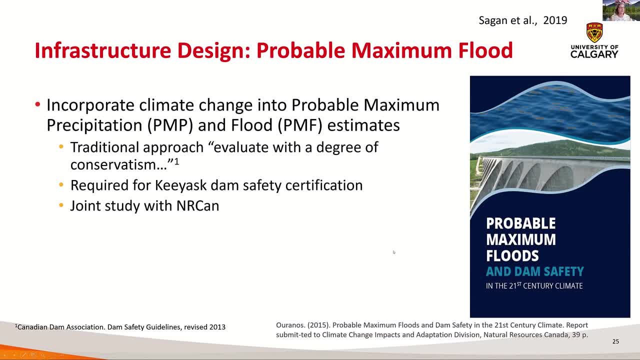 new infrastructure that was being built on the Northern Nelson river And the traditional approach would be to use conservative estimates, But we actually managed to incorporate climate change and look at rain on snow events and critical precipitation events to get a new design: flood. We also took a multi-monthly 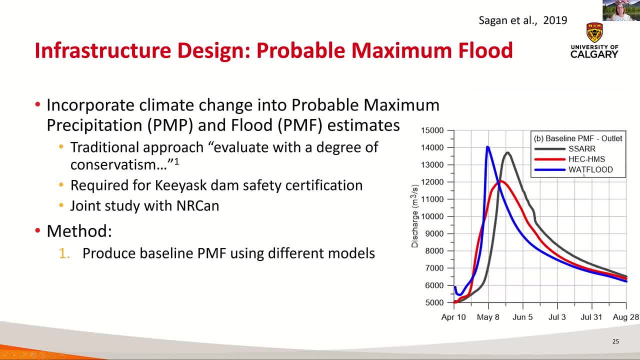 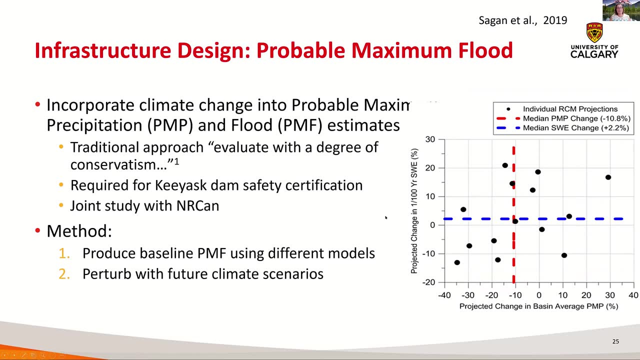 model approach to it. We didn't pick the models Manitoba Hydro did, but we used that to produce a baseline PMF from each model using their historical approach. Then we perturbed that using climate scenarios. So we actually looked at climate models and got changes in projected. 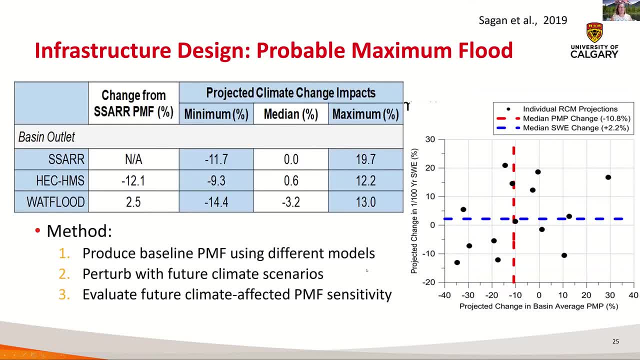 PMF. And then we evaluated that PMP sensitivity, for the PMF in terms of each model to produce a minimum, a median and a maximum output from each model, And what we could see is their SAR model was their traditional approach that they used to use, And there was quite a bit of difference here. 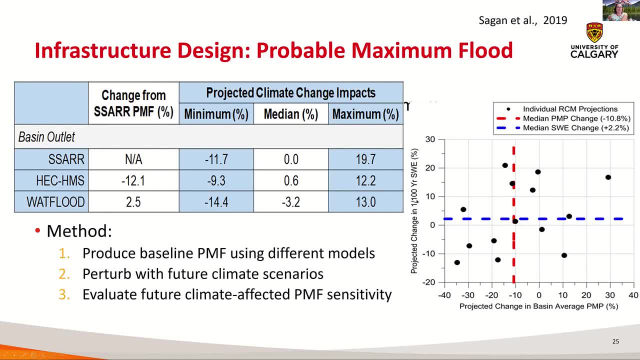 depending on which model was actually chosen, And so they did end up going with the most extreme because of the climate scenario. And then we evaluated that PMP sensitivity for the PMF. in course, we're dealing with a 500-year design life here. You don't want to risk overtopping that. 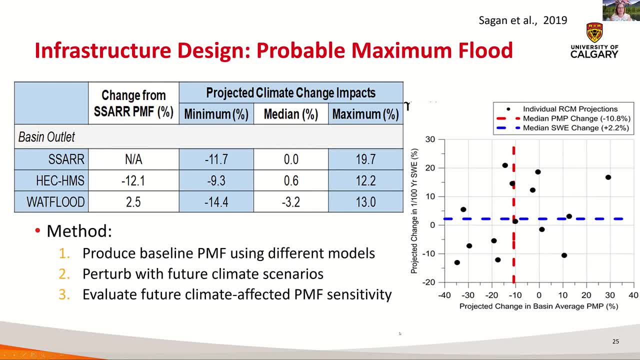 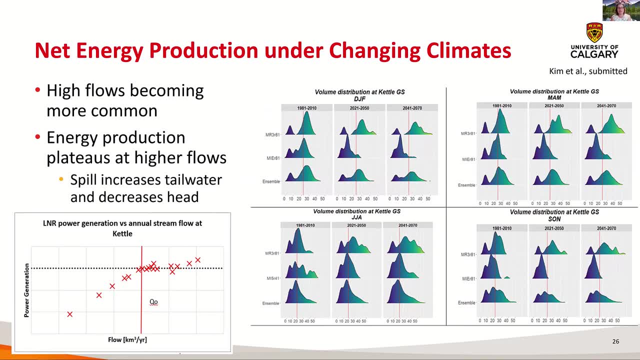 And it's better to over-design than under-design. in this particular case, We've also taken that one step further and actually looked at what the impact of these different flow scenario projections within this hydroelectric generating system is on energy production. So what we do know from the graphs on the right-hand side which are showing: 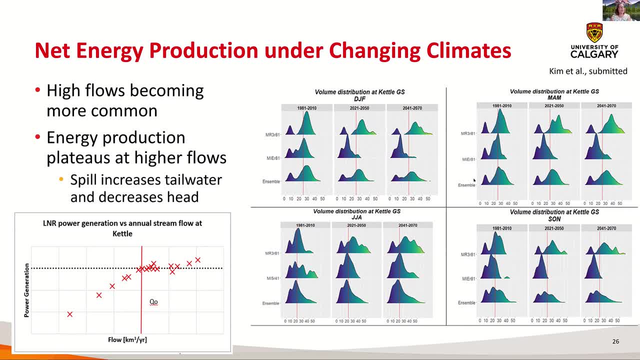 the PDFs of the data is that the PMP sensitivity for the PMF is higher than the PMP sensitivity for the PMP, And so what we've done is we've actually taken a look at some of the scenarios for flow is that high flows are becoming more common, So the red line represents the historical peak. 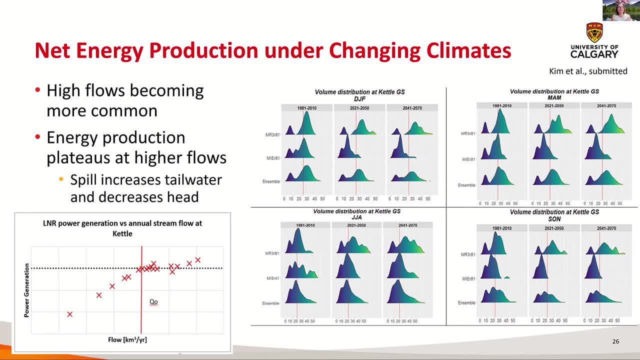 And you can see that, generally speaking, there is now a shift to the right of the red line, So there's definitely more high flows, And the question is: how does this impact energy production, particularly in the lower Nelson, where there isn't a lot of reservoirs And what you can see? 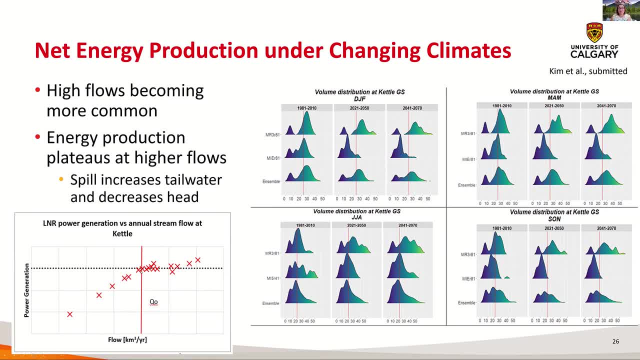 is that up to a certain threshold you will generate more power, more water, more volume and more energy. more volume, more power, more energy. But then you hit a threshold And at that threshold it sometimes goes down, or at least plateaus, And the reason for that is because you have to spill. 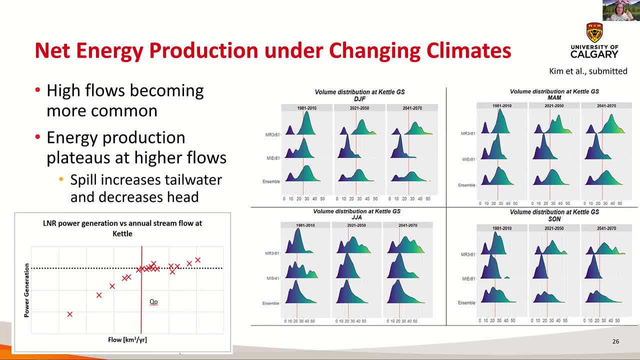 Once you exceed your powerhouse capacity, you're now spilling water. Once you do that, the difference between your headwater and your tailwater levels out and there's less of a head drop. So as your tailwater comes up, because you're spilling those two even out, there's less head. 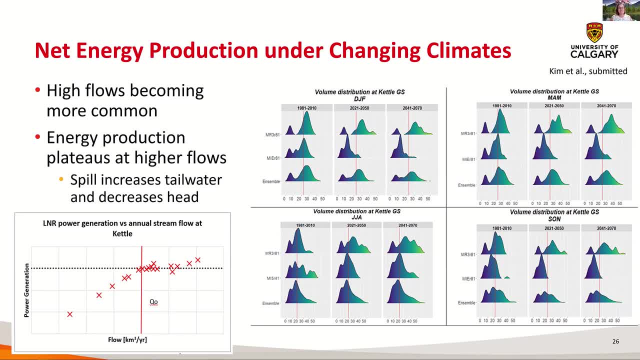 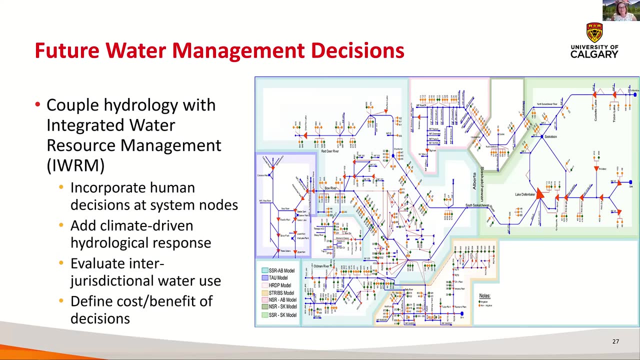 difference, which means there's less power generated, And so that's kind of a critical threshold within the Lower Nelson, because after that their systems are really inadequate and they have to look at expanding their powerhouses or changing the configuration. We've also taken that one step further and looked at the system as a whole in terms of the sum total. 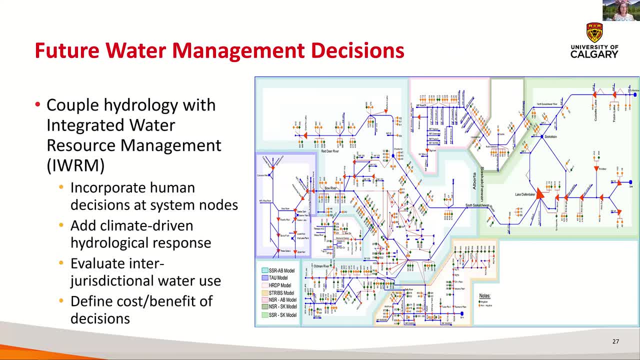 of all management decisions, not just hydropower, but incorporating everything into an integrated water resource management model. And that's what's shown on the slide On the right-hand side. it's a network diagram of every node within a system where a decision 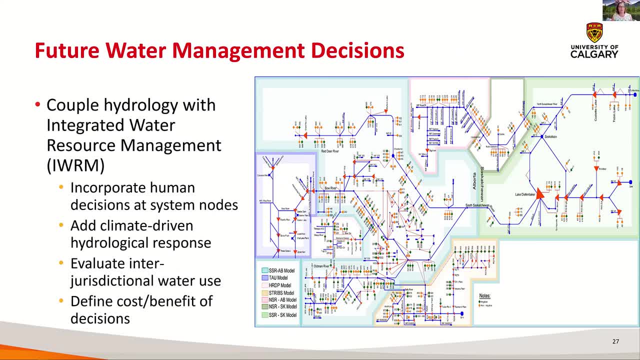 has to be made that controls the function of water, And this is showing the Saskatchewan River Basin as a whole, So everything upstream of Manitoba. We incorporate those human decisions, Then we add the climate-driven hydrologic response And then we evaluate the effectiveness. 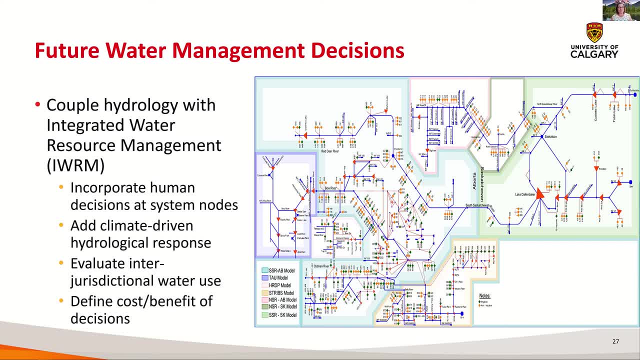 of those interjurisdictional rules to see if they're still adequate. We can also add cost benefit of future decisions. And then we add the cost benefit of future decisions. And then we add the cost benefit of future decisions. And then we add the cost benefit of future decisions. 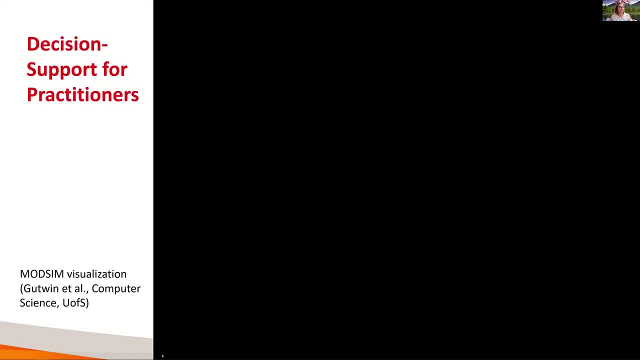 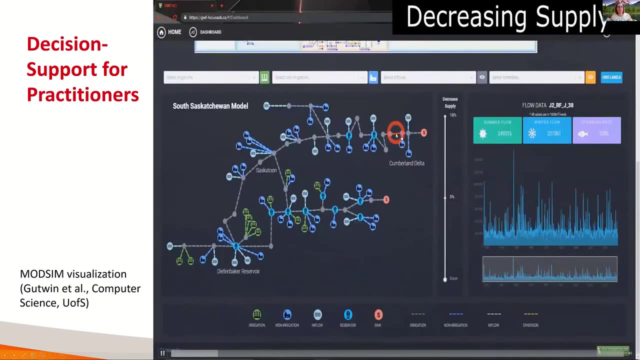 So I think I have a video clip embedded here that shows you how we take this from the network diagram to a node to look at the hydrograph over time and the environmental impacts of changing that flow scenario- a decrease or an increase in supply- And we've even got ecological decisions. 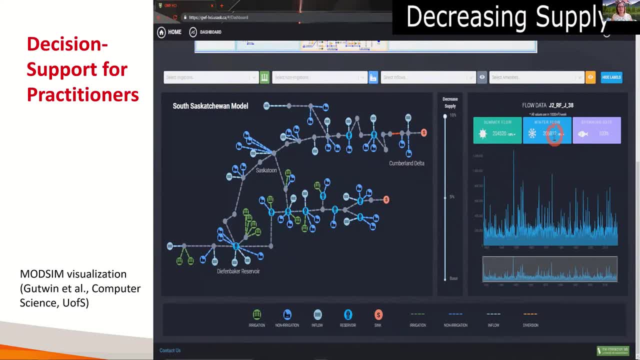 associated with water temperature embedded in that flow scenario. So we've got a lot of data embedded in this network model to look at how that might affect fish spawning, for instance. And that's just a sample of one of the decisions So we can evaluate eco-hydrological needs. 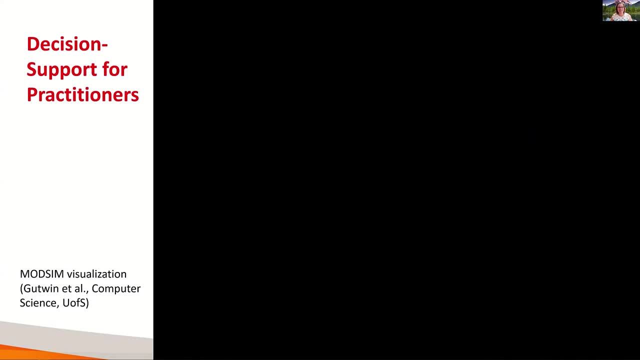 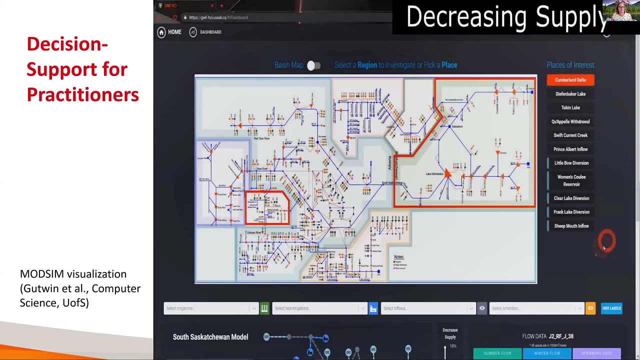 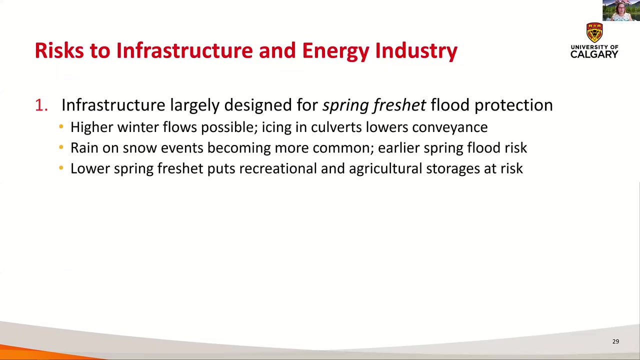 as well as economic needs, as well as hydrologic change, all as a result of climate change. Sorry, just play it again. Okay, So to wrap up here. I don't know if you can hear me. Okay, So to wrap up here. 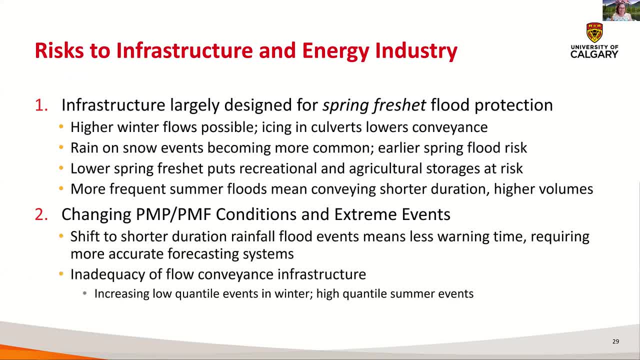 I don't know if you can hear me, Okay. So to wrap up here, the risk to the infrastructure and energy industry that we see. largely this infrastructure has been designed to deal with or protect against spring fresh set that peak flow coming in the. 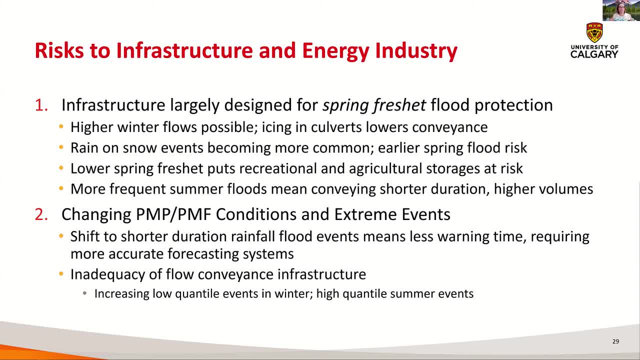 spring. What we're seeing now is a shift towards more of the shoulder seasons increasing in flow and a more uniform hydrograph throughout the year. Higher winter flows are possible, which means that there's going to be icing in culverts and critical infrastructure, preventing the conveyance of flow, And so this 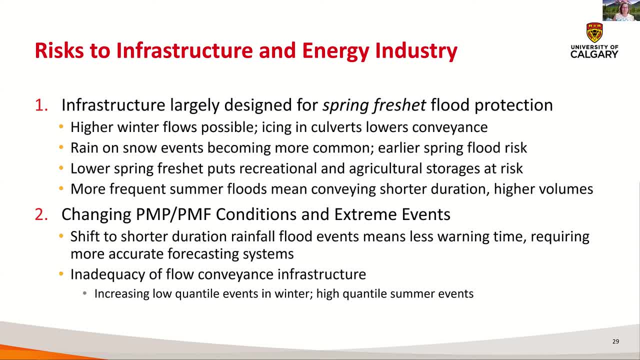 is going to increase the flooding risk. in the winter or shoulder seasons, Rain on snow events are becoming more common, which also presents a flooding risk, And lower spring fresh sets on average, because the delivery of the water is more uniform throughout the year. So that means 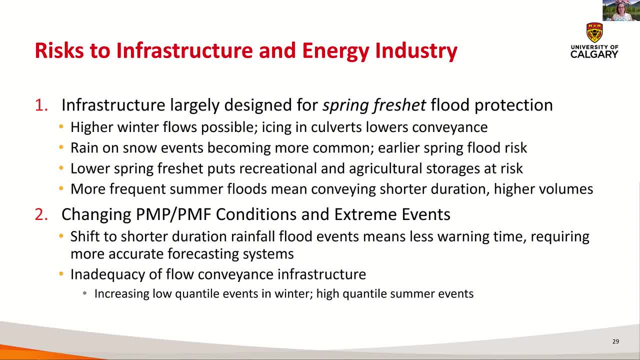 you can't rely on that to fill up your reservoirs for recreational use or also drought protection for agriculture. There's also an increase in more frequent summer floods, So we're seeing higher intensity, shorter duration rainfall events that are now occurring In 2014, for the first time ever in all. 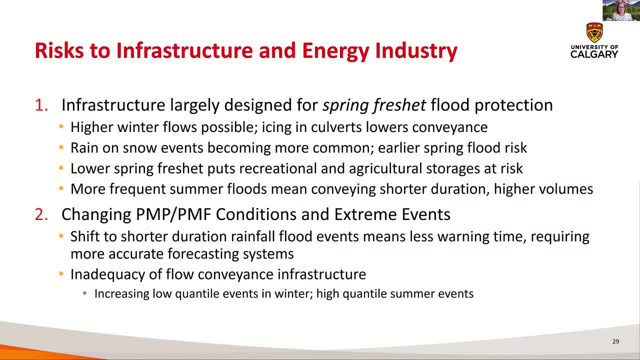 of Canada, there was a peak flood event that occurred as a result of a rainstorm as opposed to snowmelt, And that was in the Assiniboine River and it was a one in 200 year event. So it was quite significant And none of the infrastructure was prepared to handle that because the dikes 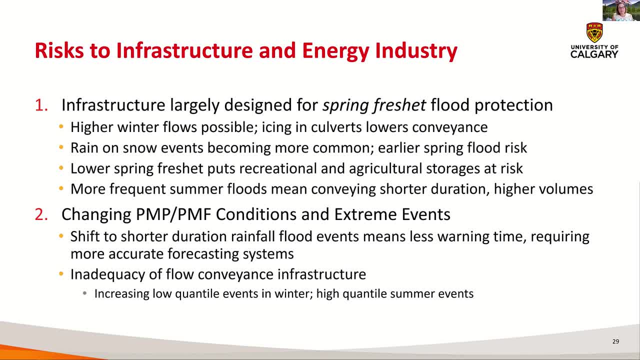 believe it or not, were designed to be frozen when the peak flows came. And they weren't because it was in July, And so it scoured the dikes and the dikes were then rendered useless. So we also have changing PMP, PMF events. A shift to shorter duration rainfall means less warning. 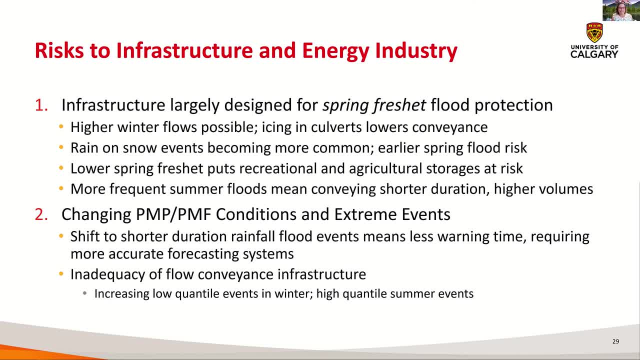 time and requiring more accurate forecasting systems and a general inadequacy of the flow conveyance infrastructure. So we're seeing an increase in more frequent summer floods And none of the infrastructure is. So we're seeing an increase in more frequent summer floods And none of the infrastructure is. 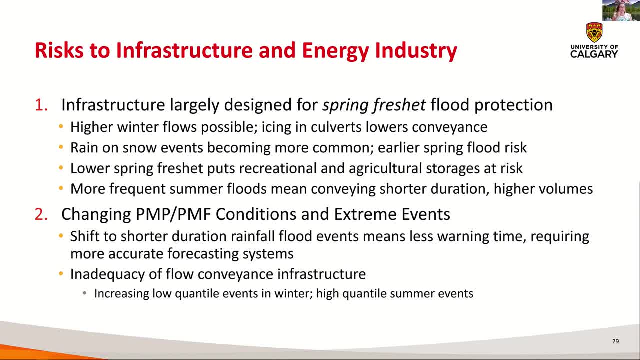 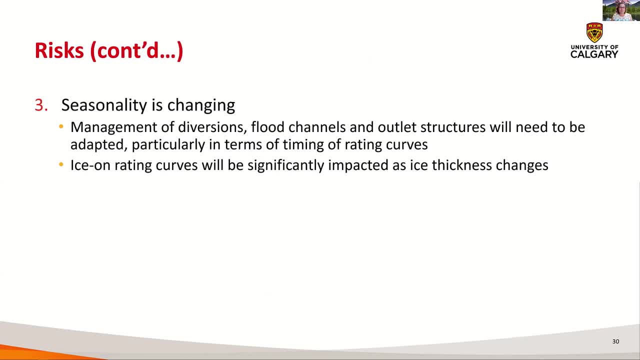 so I just talked about the dike scenario, But also looking at the increasing lower quantile events in winter and the higher quantile events in summer. Seasonality is also changing. So management of diversions, flood channels, outlet structures, hydropower- was all designed around the 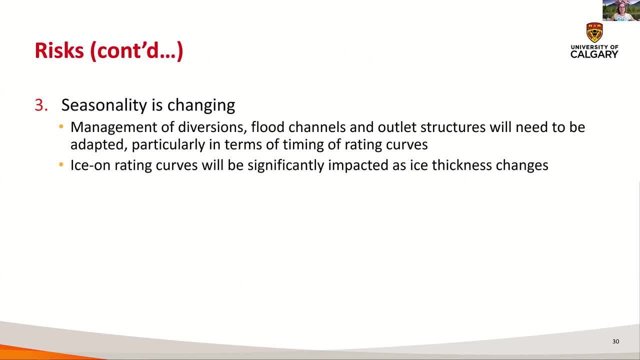 idea that we have this peak event in the spring and the rest of the year it's fairly low And of course that's now changing. And ice on reading curves, ice breakup and ice formation is becoming more critical Because it's becoming a lot more dynamic every year. Management of ecological and environmental flow. 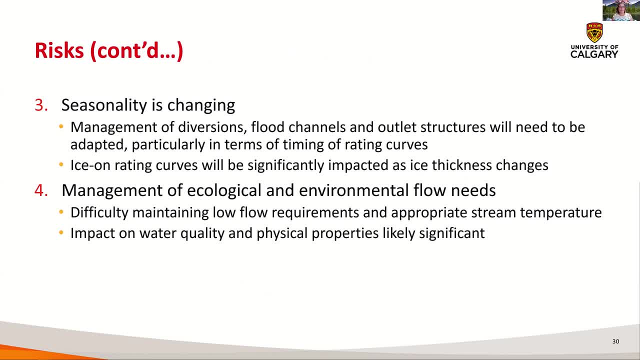 needs. there's difficulty maintaining these low flow requirements because of this rapid swing from flood to drought and the impact on water quality and things like fish spawning because of temperature and increasing long term drought risks. So the prairies are right now in approximately. 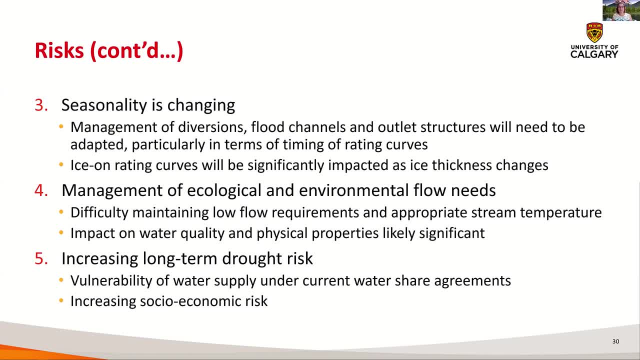 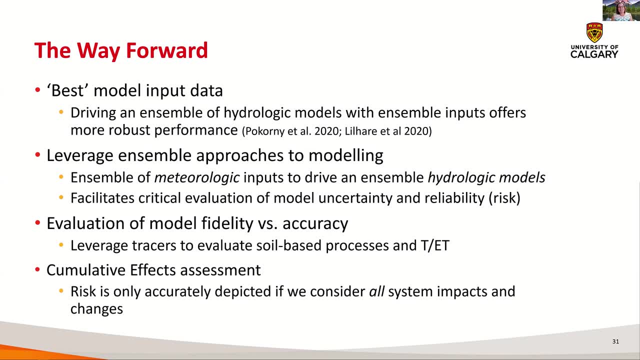 a one in 150 year to one in 200 year drought currently. So this is becoming more common. So the way forward, what my group is working on under Abbey Nets and beyond, is ensemble based approaches, to put it mildly. So driving ensembles with ensembles. So there's no such thing as one best input or one best output, but really leveraging those ensembles to do more accurate uncertainty analyses. 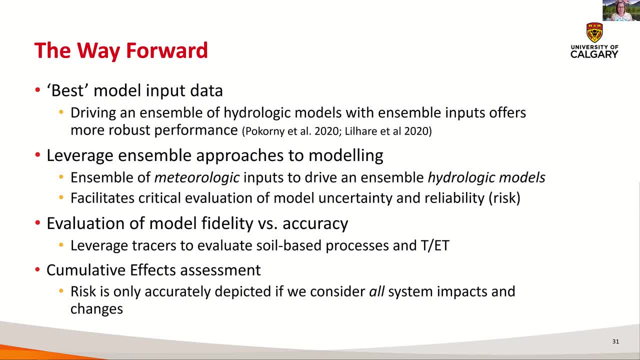 And certainly making sure we're getting the water in the right place. not just total stream flow, but looking at water on the landscape and cumulative effects assessments, So taking it beyond just hydrologic change or climate change but looking at ecological and economic impacts as a result and looking at that as a whole, not one system in a silo, but developing models that are capable of looking at this simultaneously. 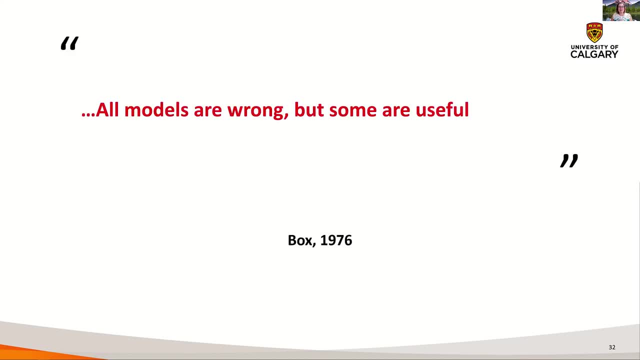 My end quote: all models are wrong, some can be useful, And that's it. That's all I have for today, So happy to take questions, comments and discussion.